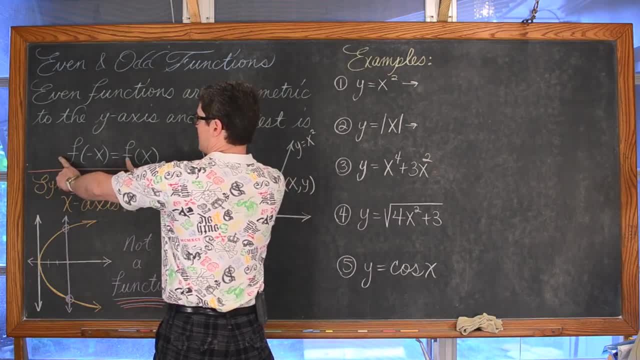 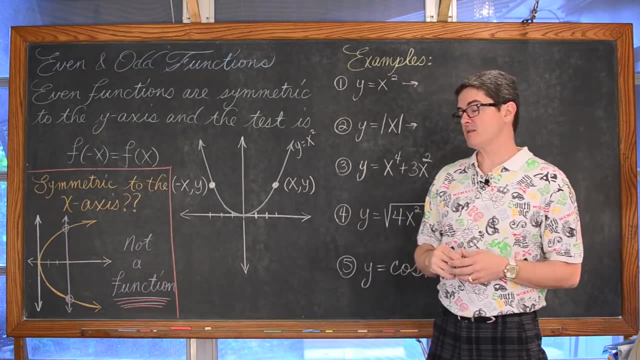 test is: when you plug in opposite values, you get the same answer. These are the same names on both sides. There is not a 2 here and a 1 there, so we are getting the same answer. That is what algebraically that says. Graphically it is like this parabola that 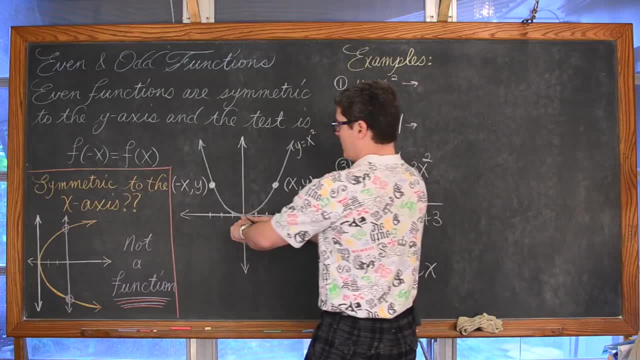 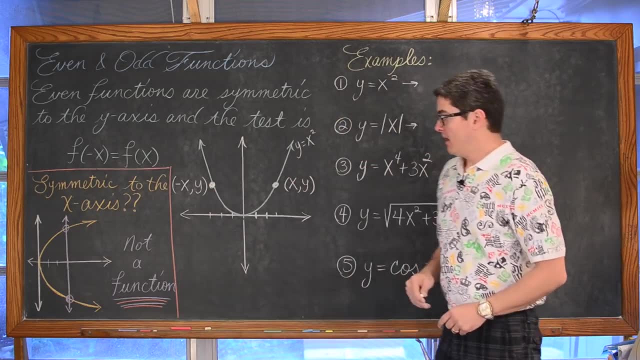 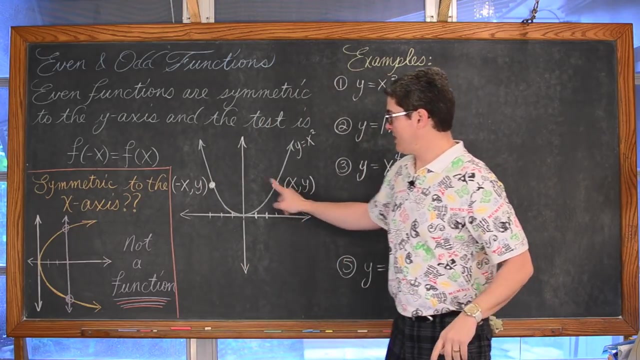 we have here, y is equal to x squared. When you plug in opposite values, you get again the same answer. So like negative 3 squared is 9 and positive 3 squared is 9.. So you have this reflection, this symmetry over the y axis. You get that graphically by the fact. 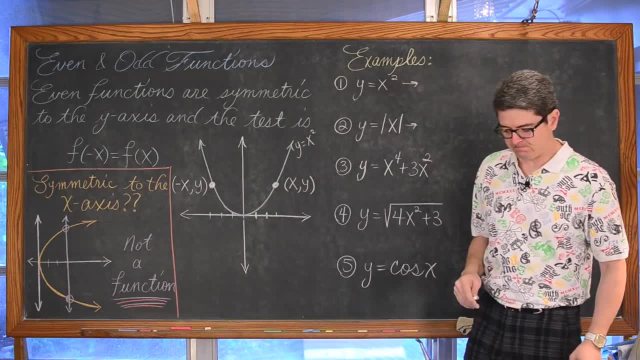 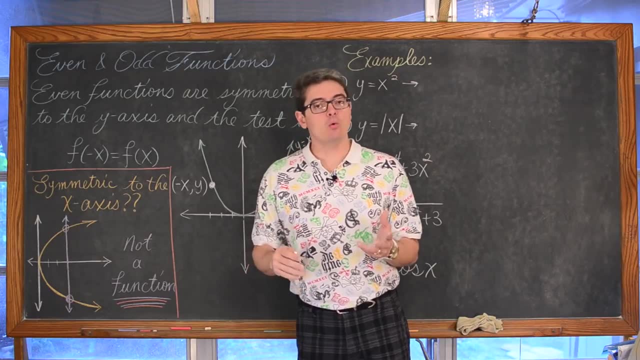 that we have the same y value but opposite x's. So I just mentioned symmetry to the y axis. When we get to odd functions, I will be talking about symmetry to the origin. What you will not hear me talk about, other than the fact that it is incorrect, is symmetry. 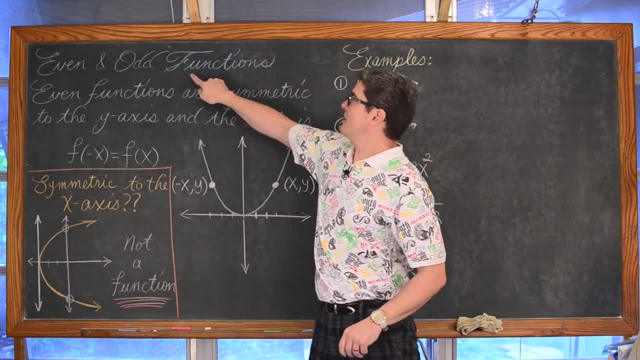 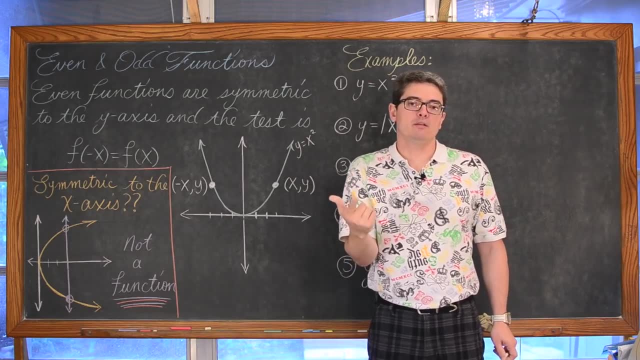 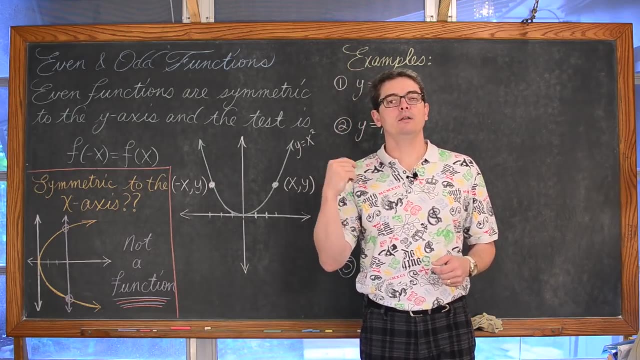 to the x axis. We are talking about even and odd functions. A function, something where every single element in the domain, or every independent value, or every x value, if you want to get less technical about it, is only matched up with one y If we are saying independent. 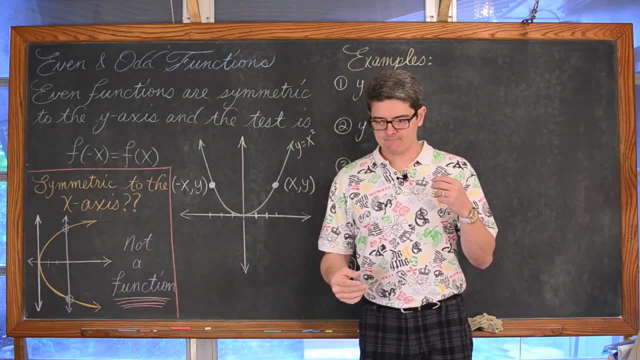 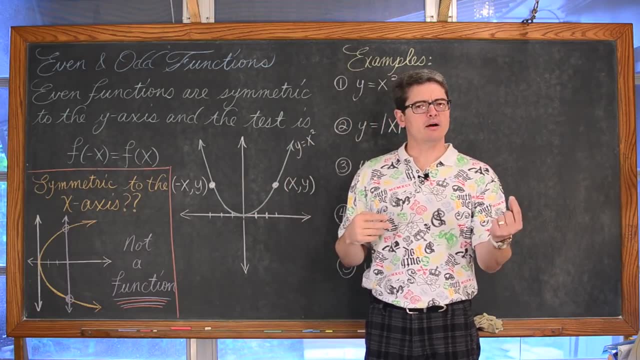 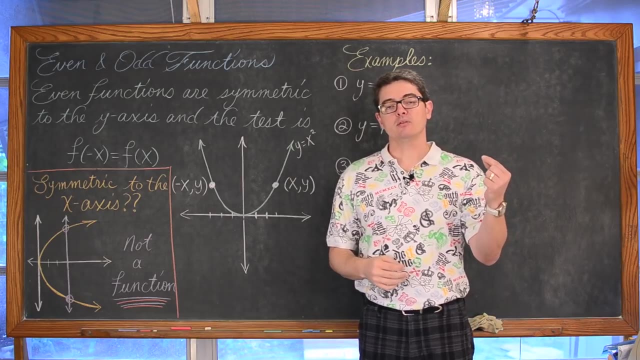 one domain value. If we are saying domain- excuse me- one x to one y, one independent value to one dependent value- I was not sure if I said that right- and every one element in the domain is matched up to only one element in the range. I am saying the same thing with 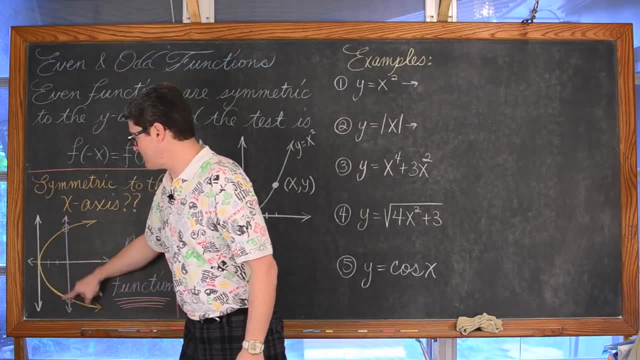 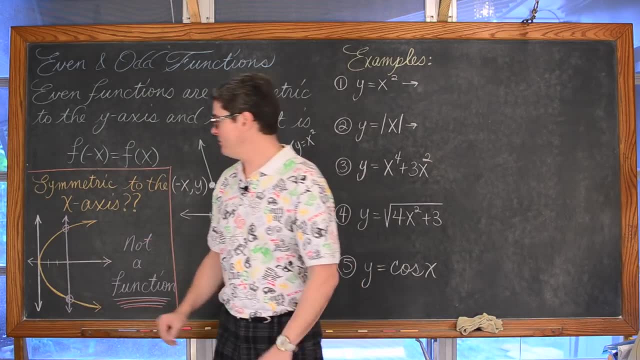 different vocabulary. So if you have an equation that is symmetric to the x axis, that means that it would fail the vertical line test. When you drop a vertical line representing an x value, if it can cross more than once, well, it is not a function. 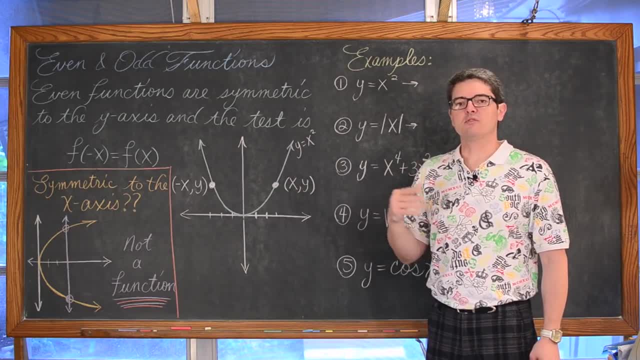 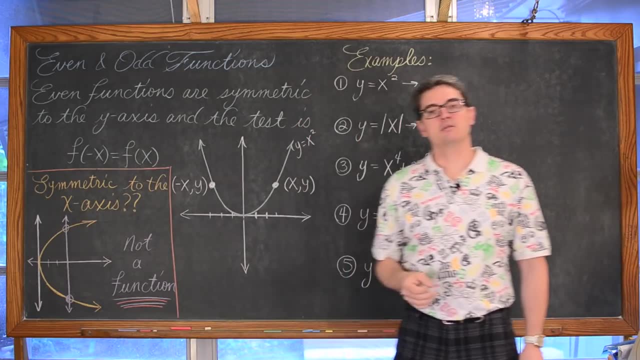 it is a relation, So we are not talking about types of relations, we are talking about types of functions. Thus we will- other than right now, where I am saying it is incorrect, we are not going to be talking about symmetric or symmetry to the x axis, So we have some. 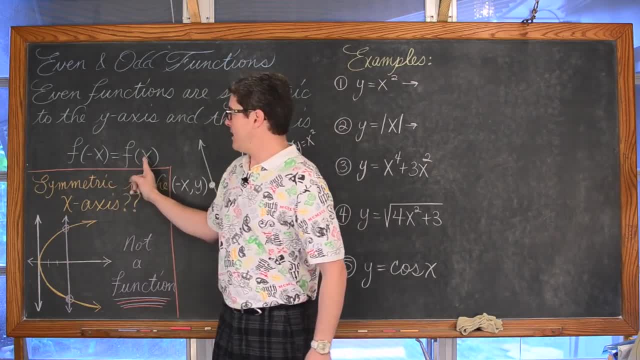 five examples here which I want to discuss with you. We are going to algebraically check whether they are even or odd. If you have a graphing or are allowed to use a graphing utility, of course you can graph it and just see that. 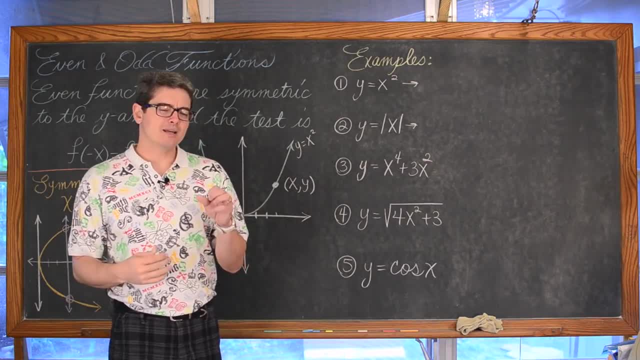 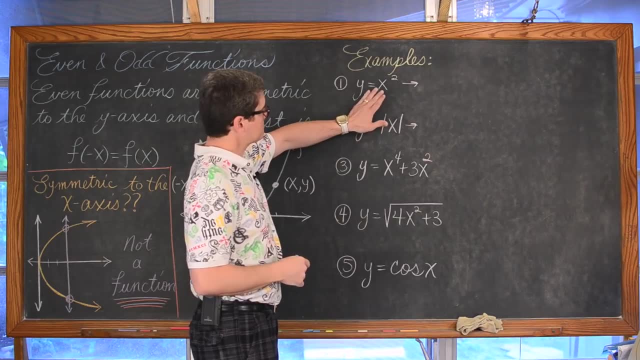 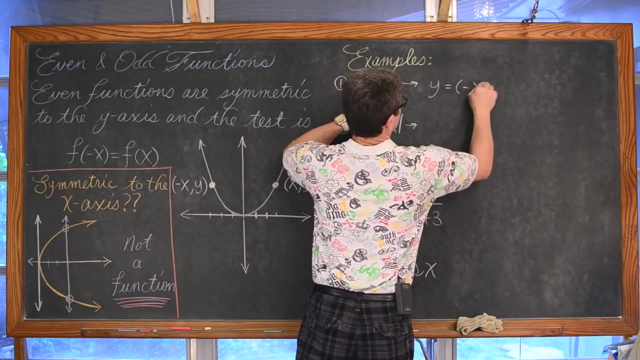 symmetry to the y axis. But graphing utilities cannot show holes in the graph. They can just sometimes be a little bit misleading. So we would like to be able to check algebraically: If we have y is equal to x squared, then we can take this plug in the opposite of x. 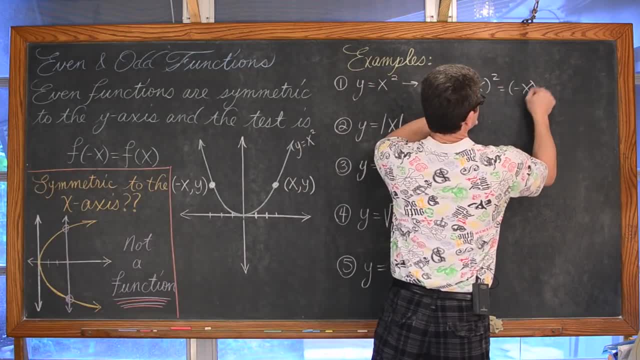 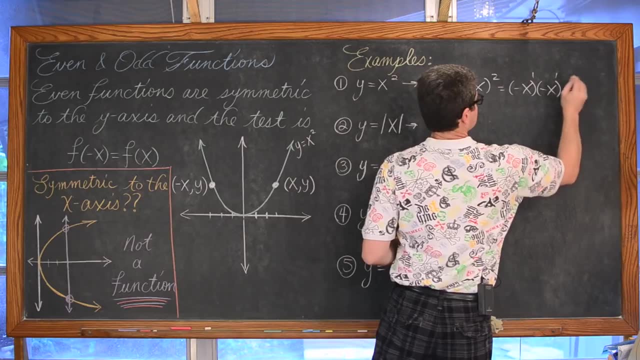 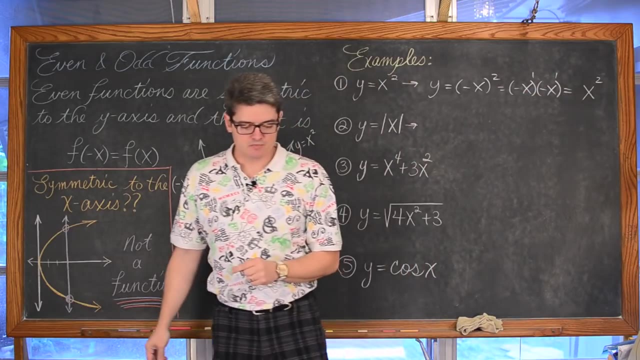 and get that negative x Times negative x. See, I am saying negative again. Those two negatives or those two opposite signs are going to cancel each other out. We are going to get x squared Because when you multiply like bases, you add those exponents. Please note that I wrapped that in parenthesis. 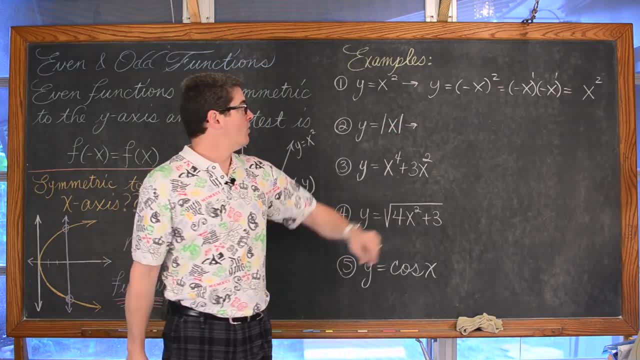 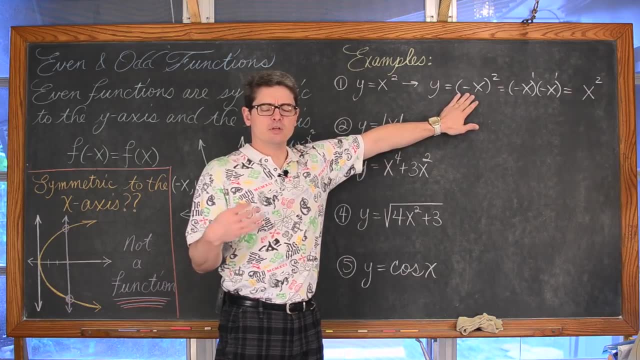 Every time you do substitution, you should be putting parenthesis around where any of your variables used to be, so that you can correctly get your signs correct Or maybe even apply the distribution. So you can get your signs correct Or maybe even apply the distributive property correctly if you happen to have substituted in an expression, Because 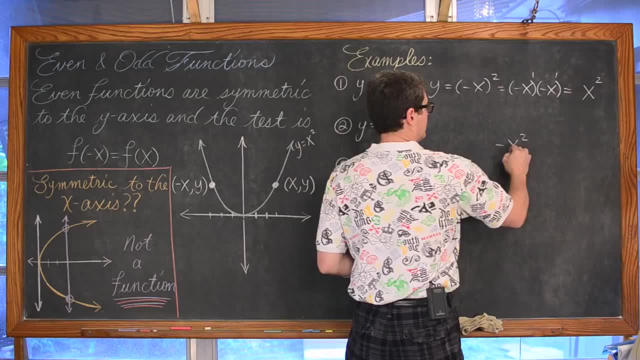 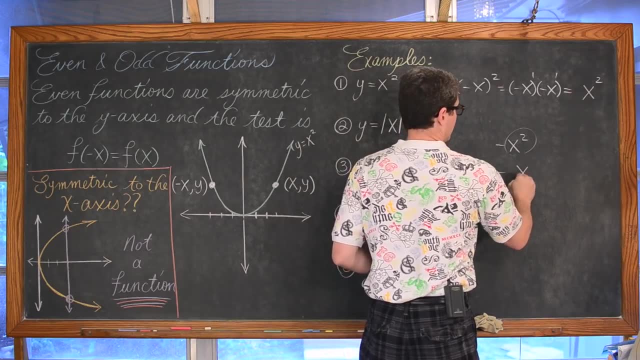 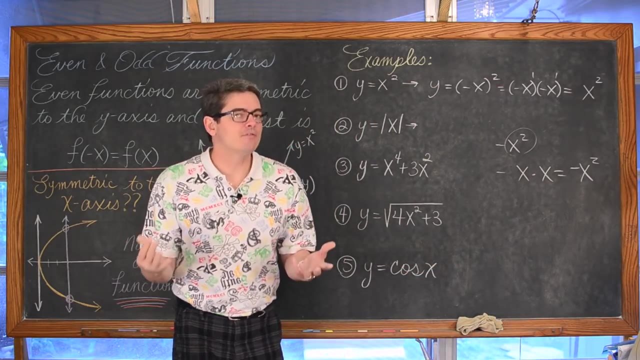 if I had wrote negative x squared. well, the only thing that that power of 2 is acting on without parenthesis is the x, And that would be negative x times x, which is negative x squared, Which, of course, I mean we can have functions that are even or not even. 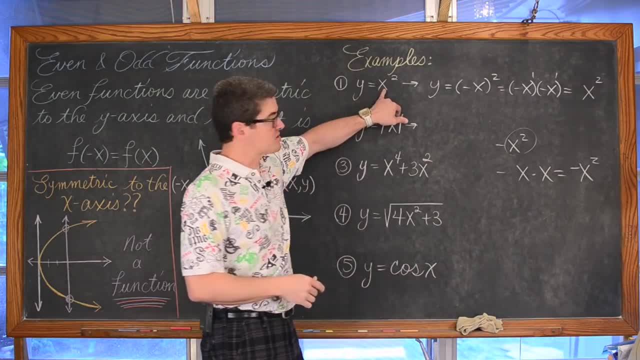 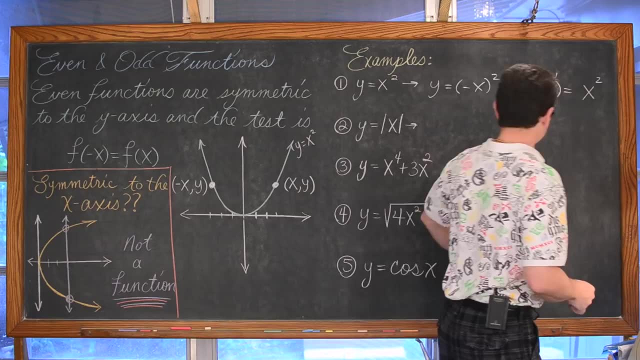 But that, in this particular case, is an incorrect answer Starting from here. So we are going to go back to the first one. We are going to substitute in the opposite of x: Okay, I need to harp on that all the time with my students, because they always forget to use. 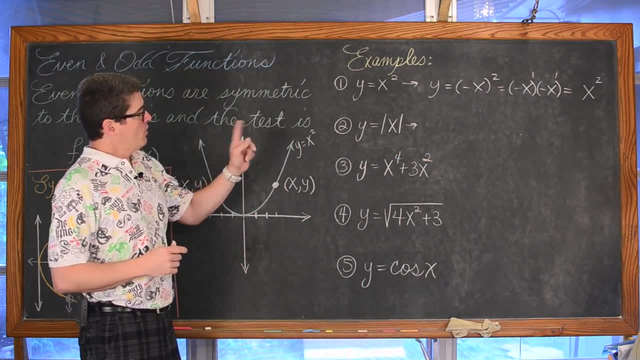 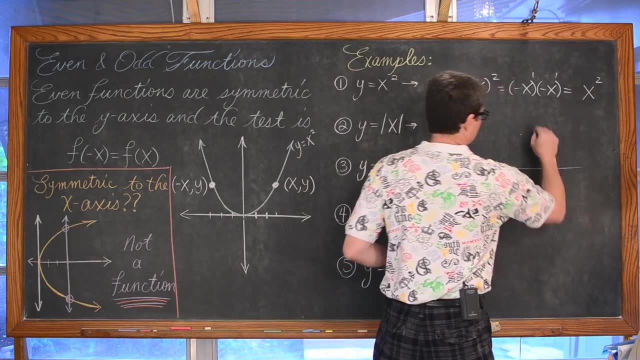 parenthesis when they substitute, We have: y is equal to the absolute value of x. Now if you know what that, what we call parent function- looks like, then you will already know that this is an even function. It is basically kind of like a v with the sharp. 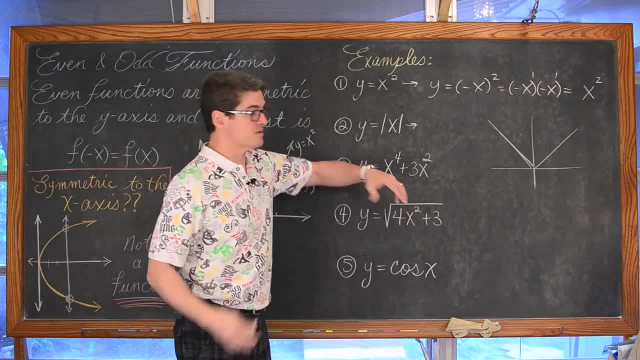 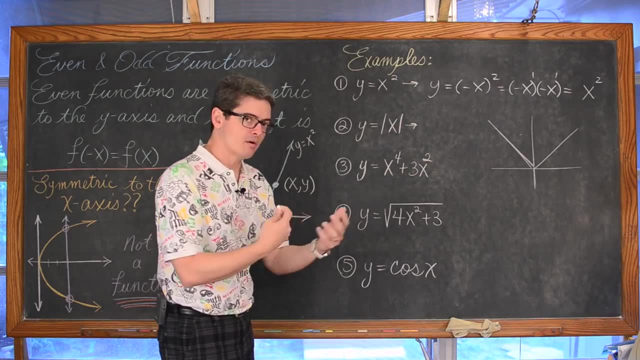 bend on the origin. It is at zero. zero because, or it is at the x value of zero, because the The x value of zero makes the expression inside the absolute value symbol equal to zero. That's where your sharp bends occur in absolute value graphs. 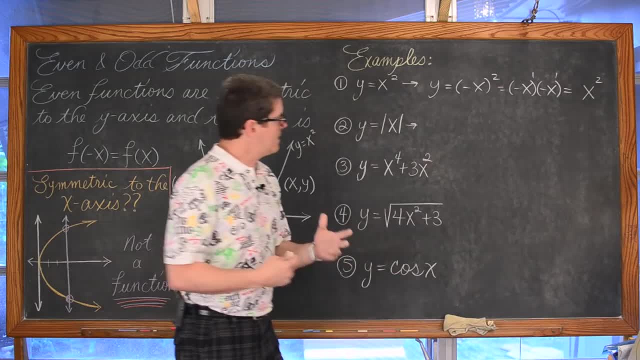 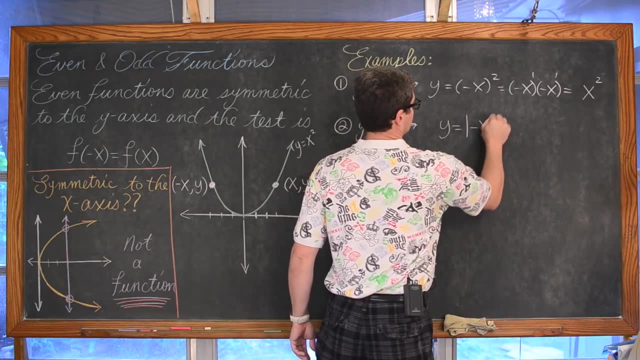 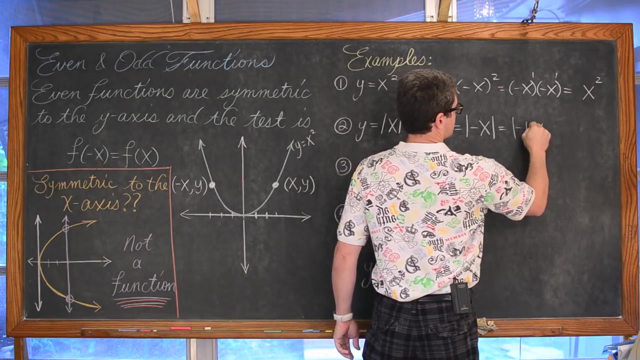 And algebraically though, how you can test with this notation of plug in the opposite of x. well, this becomes: y is equal to the absolute value of the opposite of x, which you can think of as the absolute value of negative one times x. 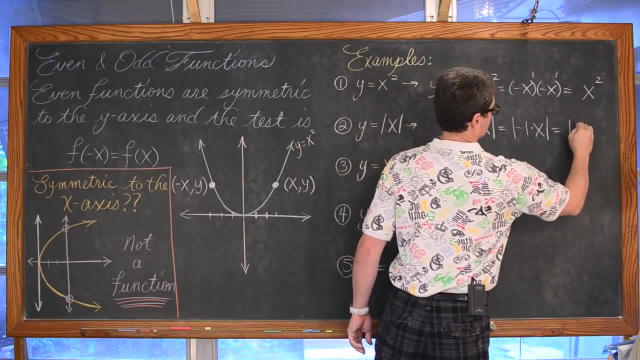 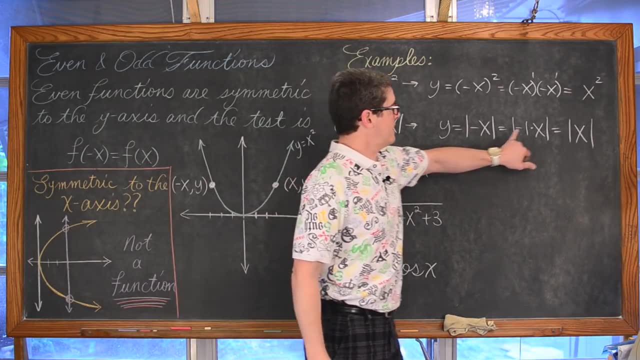 And we can take care of the absolute value of that negative one and just say: the answer again is simply the absolute value of x. So the absolute value of negative x is still going to be x, just like we started off with. So thus that is an even function. 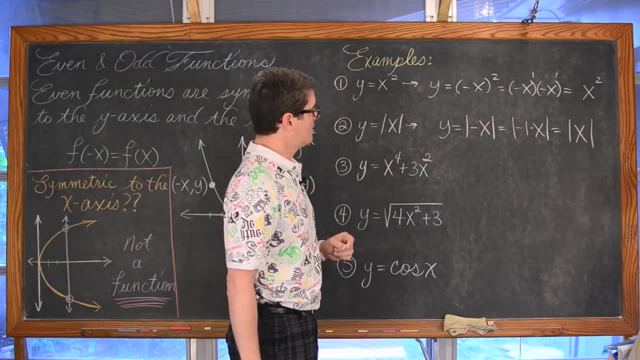 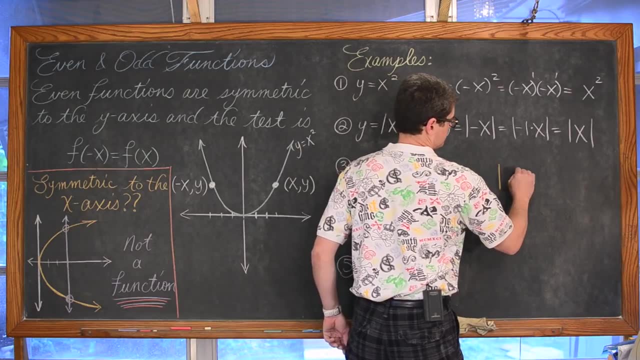 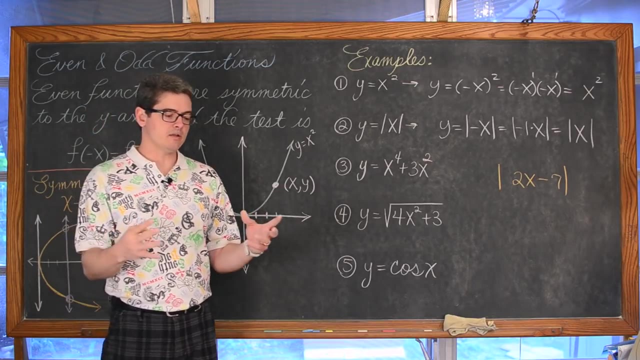 Now cautionary note here: If there are two terms in that equation- The absolute value equation or function- Then you can't just sort of like You know we do. The absolute value symbols tell us it's a function which tells us how far a value is. 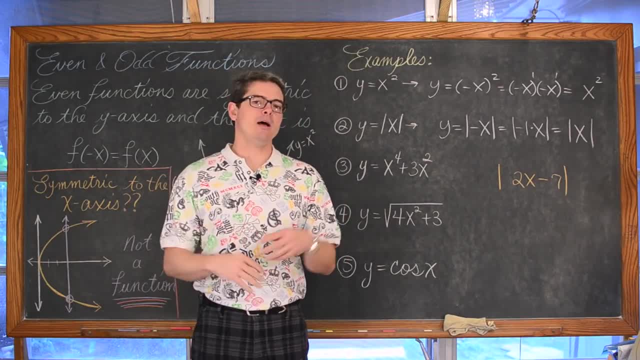 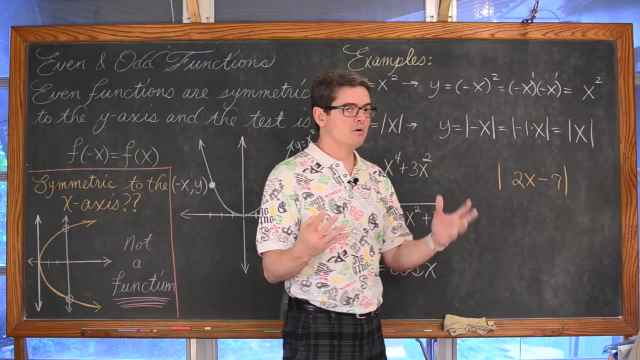 away from zero on the number line. That kind of gets short cut into: ah, it just gets rid of the negative sign. The absolute value of negative five is five. Well, that's true, but when you have two or more terms in your algebraic expression, that's. 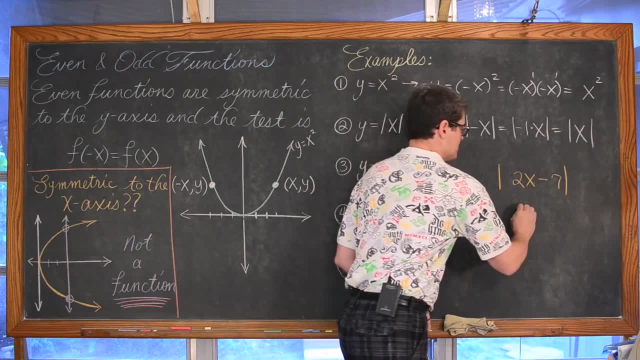 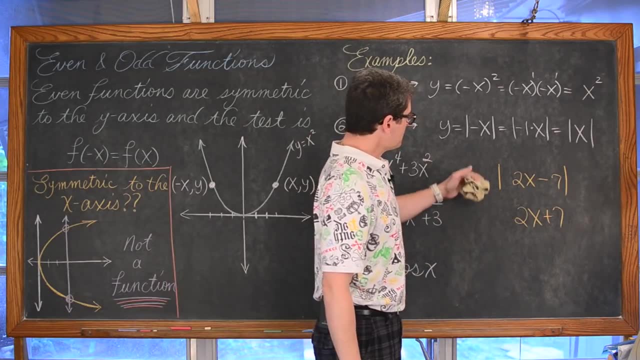 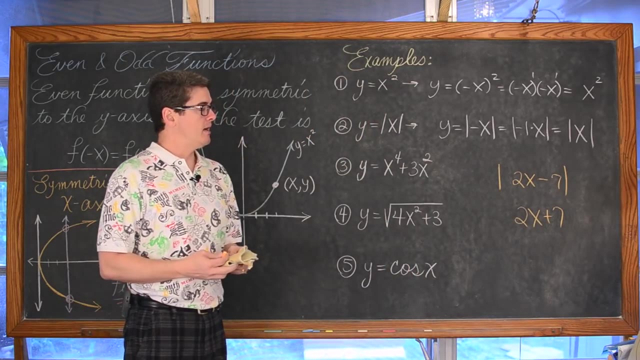 inside that function, looking at that and going, oh well, that's just Two x plus seven. That is not a correct answer. When I looked at this negative x and I showed that the absolute value of negative x was the same as the absolute value of positive x, well, for one thing, there was only one term. 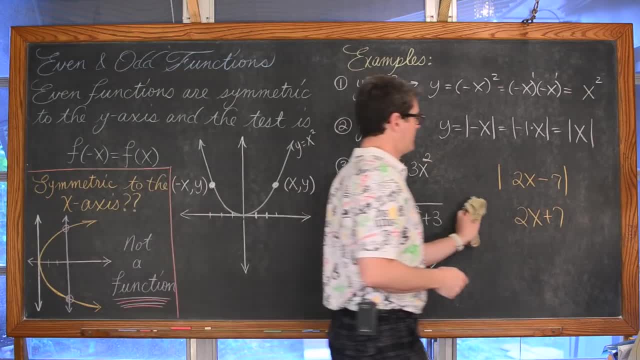 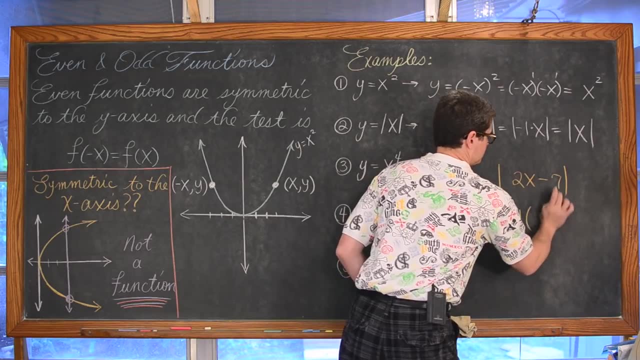 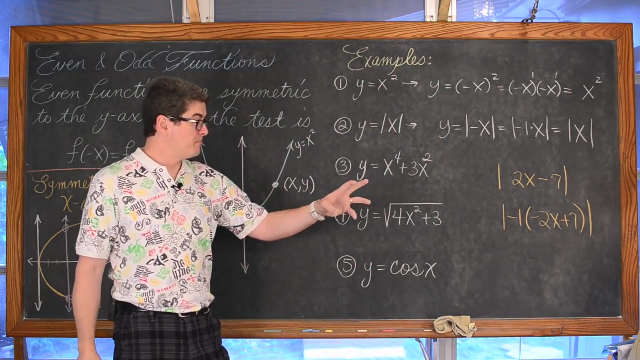 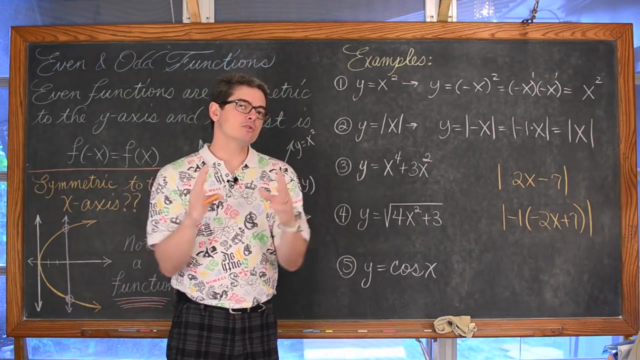 inside that absolute value function, not two. Now we could factor a negative one out. Okay, Now I'm not going to take that negative one and just sort of like, let it pull out of the absolute value symbol. They look like parentheses, but parentheses are just a grouping symbol. 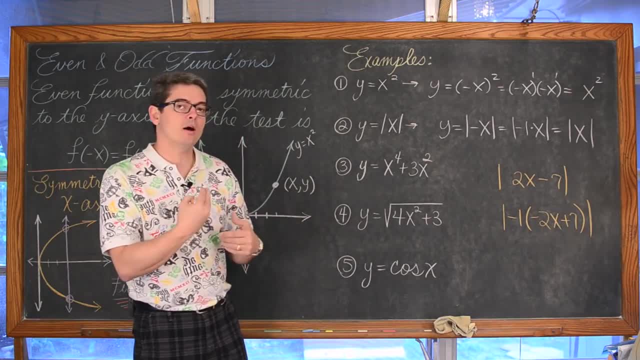 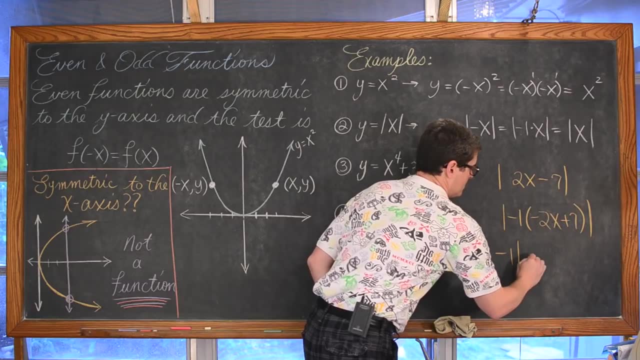 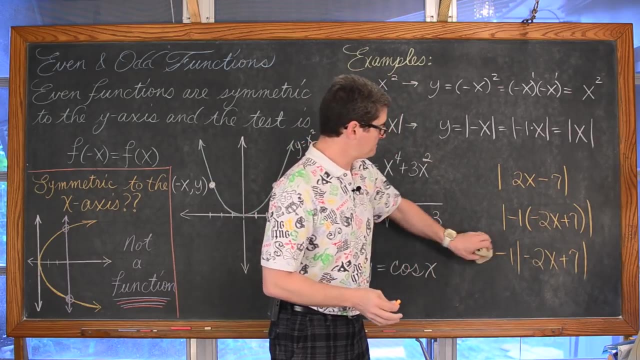 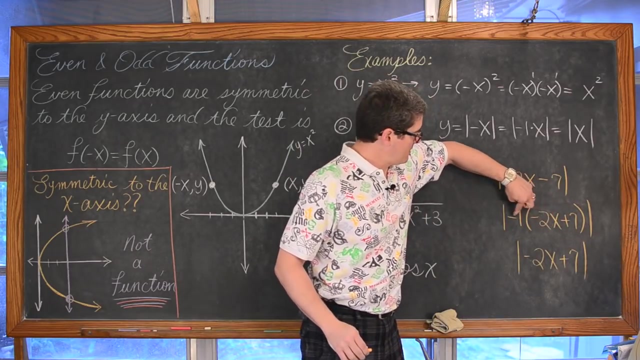 An absolute value function that they're actually doing something. Again, they're telling you how far a value is away from zero on the number line, So I can't pull the negative one out front. That would be absolutely a wrong answer. But I can recognize that, with all of this written as one single term, that the absolute 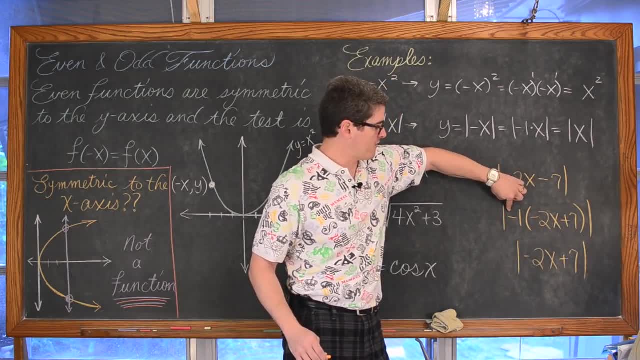 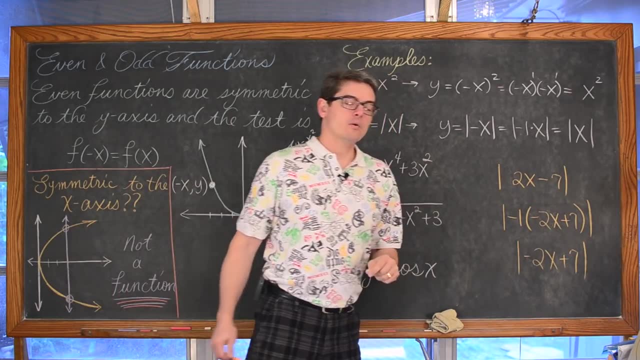 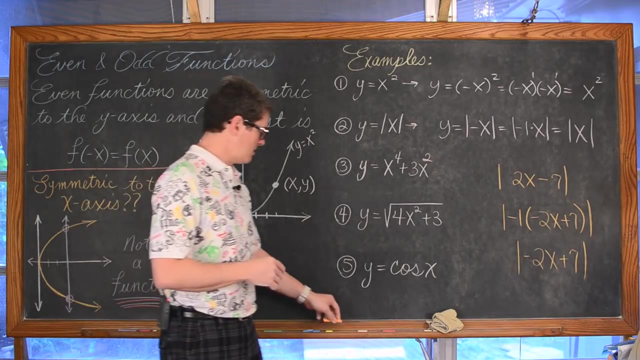 value symbols will take care of that factor of negative one out front and leave that negative two x plus seven inside the absolute value sign. These are, if you graph these, going to be equivalent or equal same graph. So absolute values can be a bit more tricky than most of these other things. 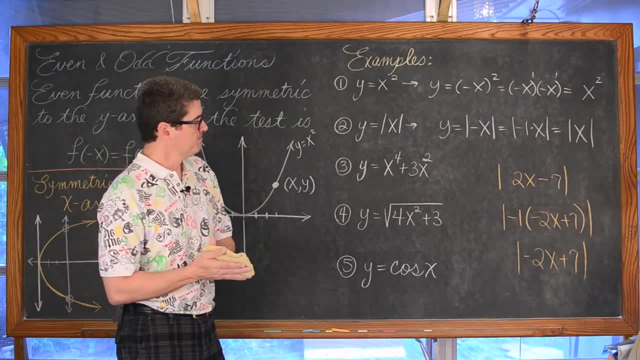 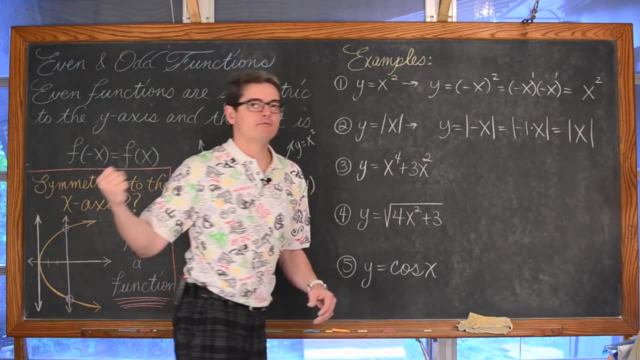 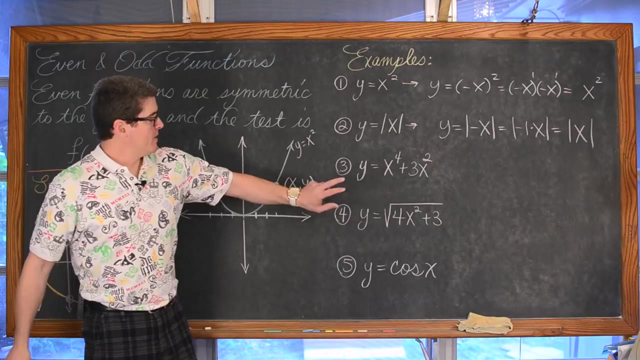 These are functions we deal with in our algebraic studies. Okay, So you can't just cancel out the negatives when there's more than one term And you cannot factor out a negative and bring it out in front of an absolute value symbol. Now here we have just a polynomial: y is equal to x to the fourth plus three x squared. 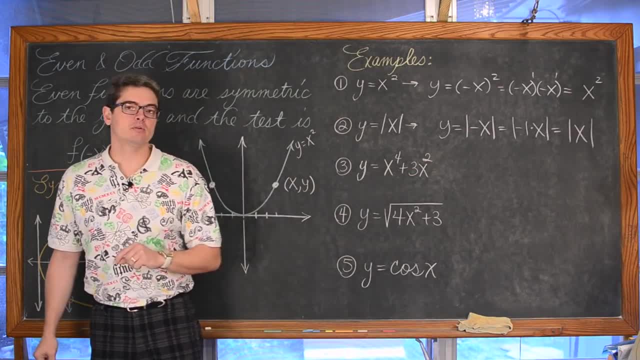 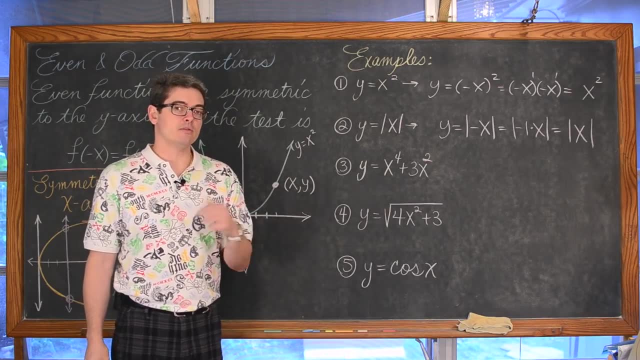 It's a polynomial because there's only one independent variable and all of the exponents are positive integers, And identifying even and odd polynomials is pretty simple too. If all of the exponents are even, it's even, And if all of the exponents are odd, then it's going to be an odd function, even though. 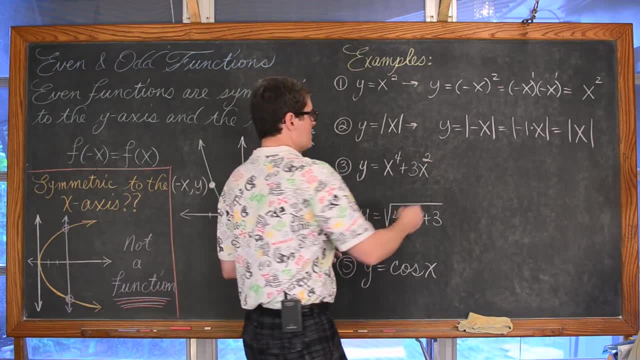 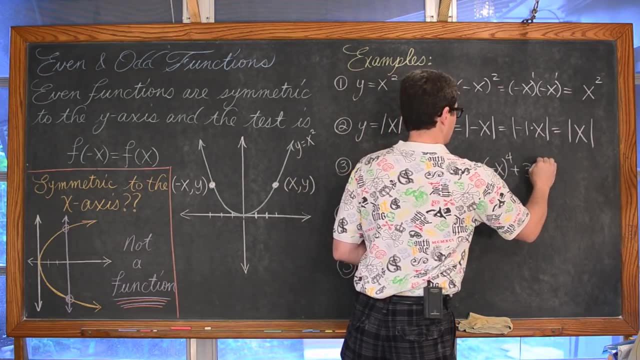 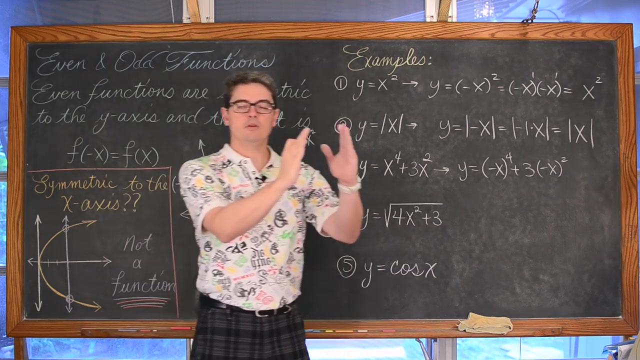 we haven't talked about odd functions yet, But again, applying the test, it's going to be: y is equal to the opposite of x raised to the fourth plus three times the opposite of x raised to the even power of two. And again, if you have an even, 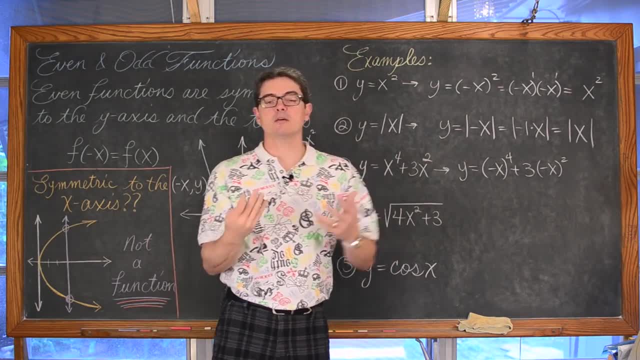 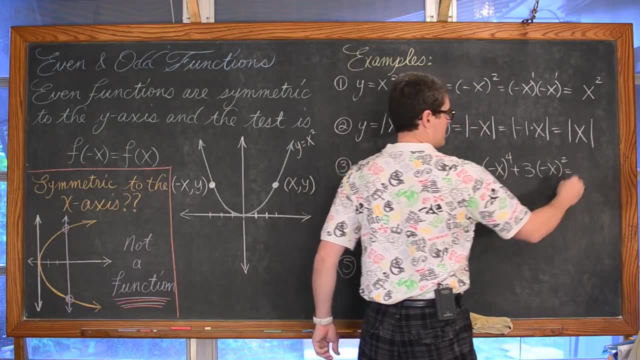 If you have just a bunch of pairs of negatives- Right Negative times, negative is positive, And so if you have a bunch of pairs of two, they're going to cancel out And this becomes- I'm running out of space here- x to the fourth plus three x squared. 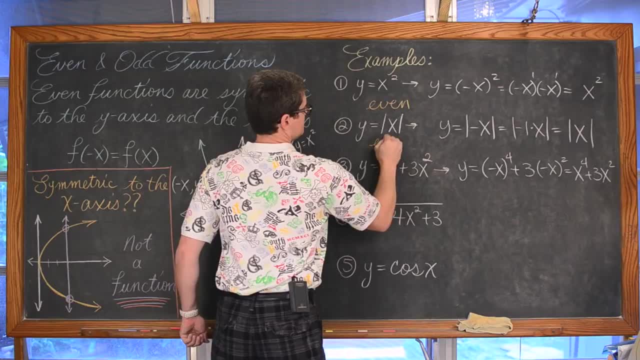 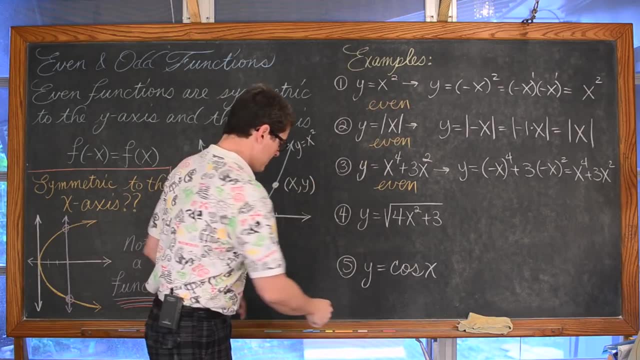 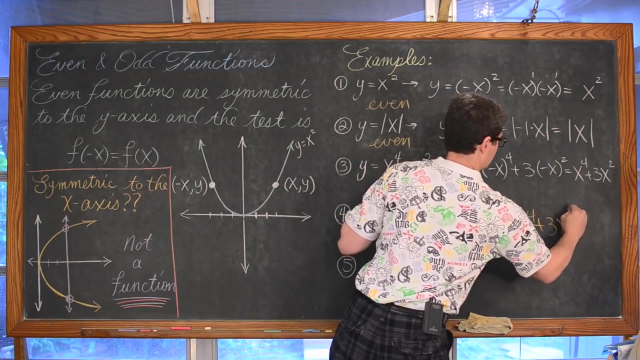 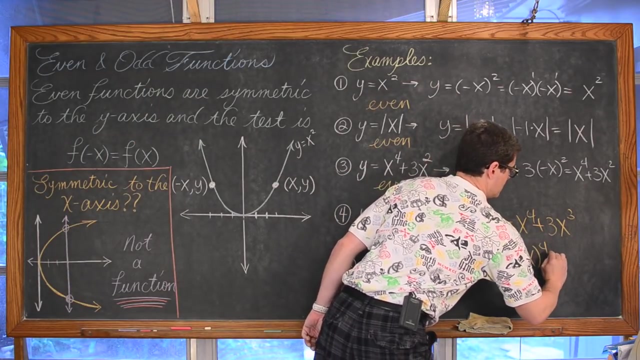 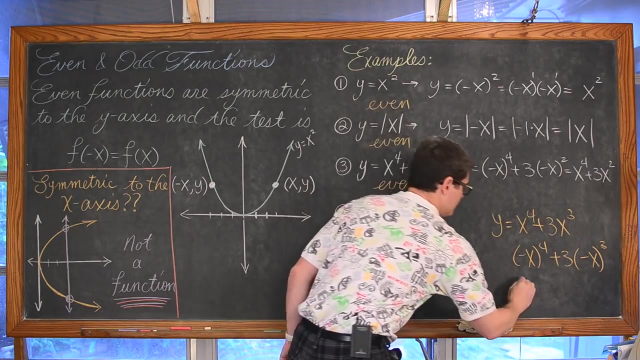 So so far, everything we've looked at has been an even function. Now what if I brought this out and said: well, this is my problem When I plugged in my opposite expression for x? well, this even power would take care of that negative. 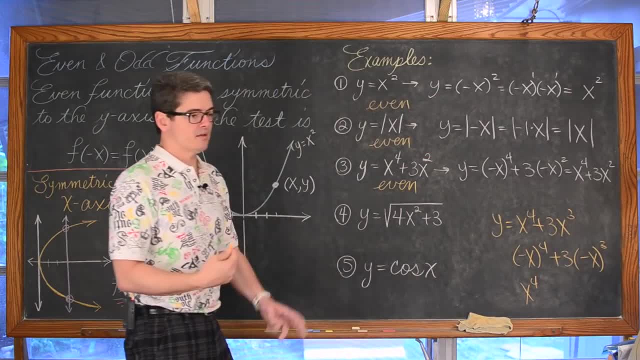 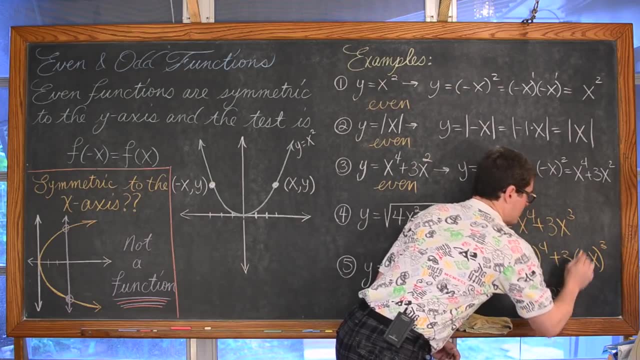 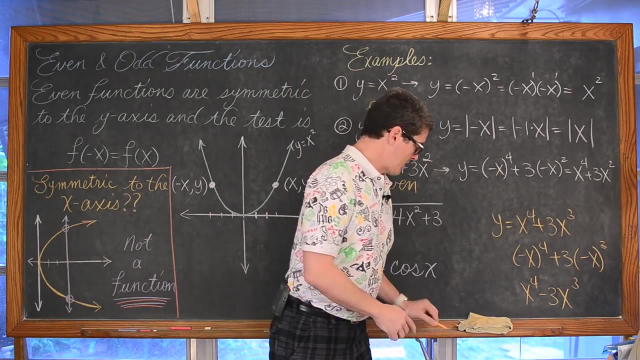 But here there's three of those negatives, So the first two will cancel out to make a positive answer. But then you bring in that one last negative sign and we'd be negative three x to the third power. So this new expression is not exactly the same as what we started with. so it is not. 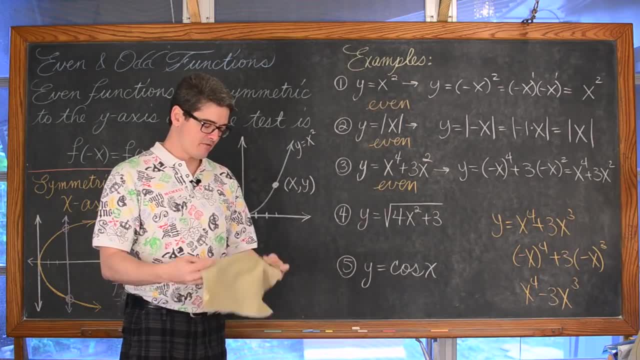 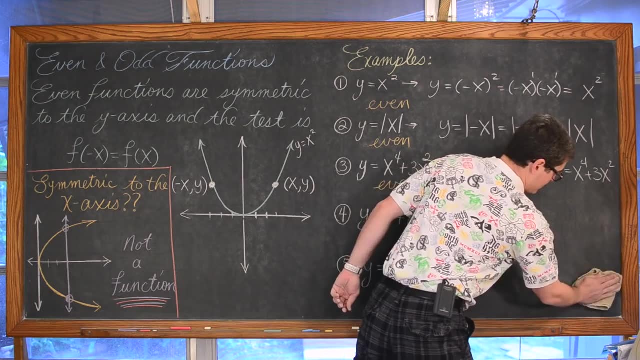 an even function, And again, we haven't gotten to the odd ones yet, but it's not going to be an odd function either. These are kind of special cases. Not most equations or functions are not going to be even or odd, But if we can identify when they are, again we can save ourselves some time. 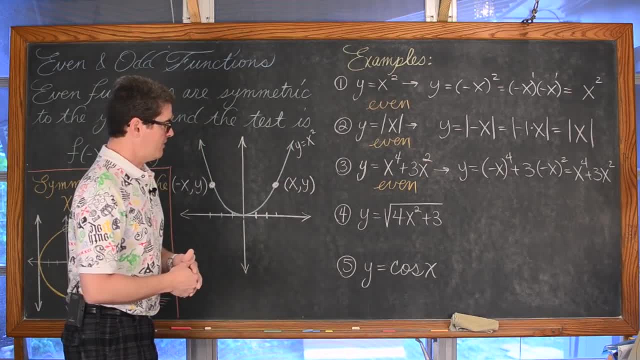 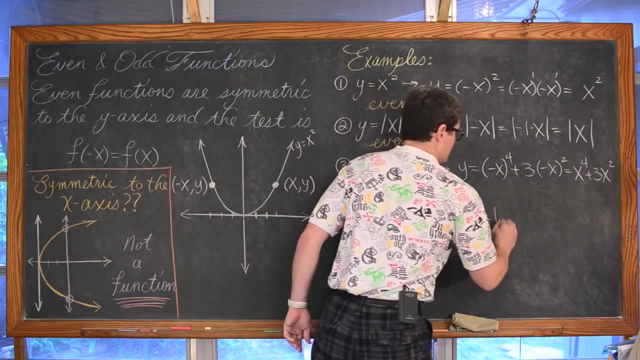 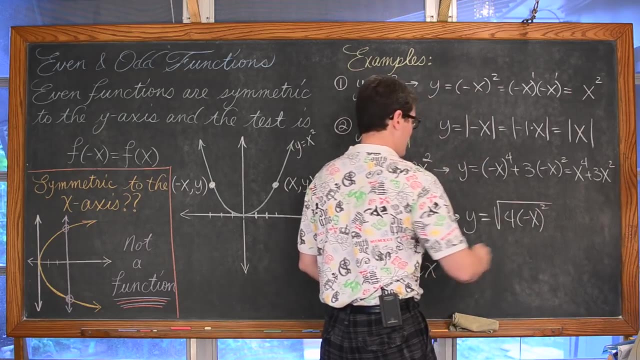 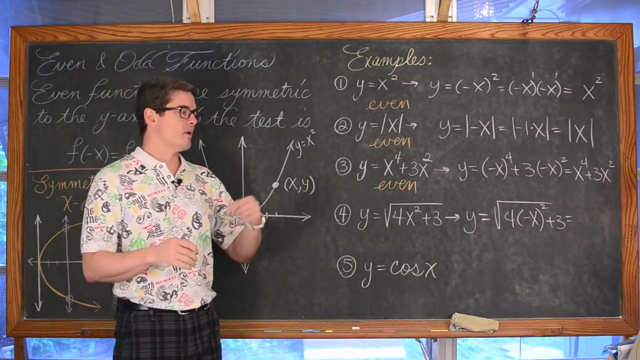 So we can certainly have a situation where it's neither even nor odd. Now here, Okay, We have: y is equal to the square root of four times negative x to the second power plus three. And again that opposite of x, that negative x being raised to an even power, that even. 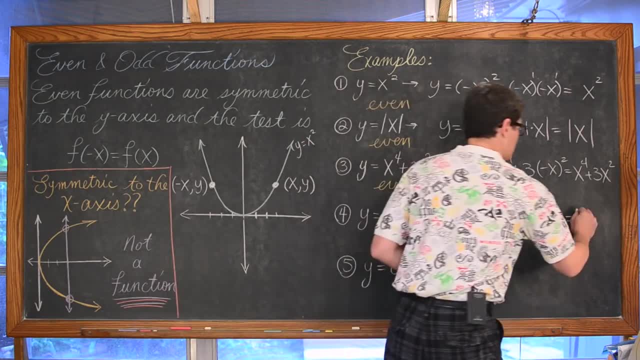 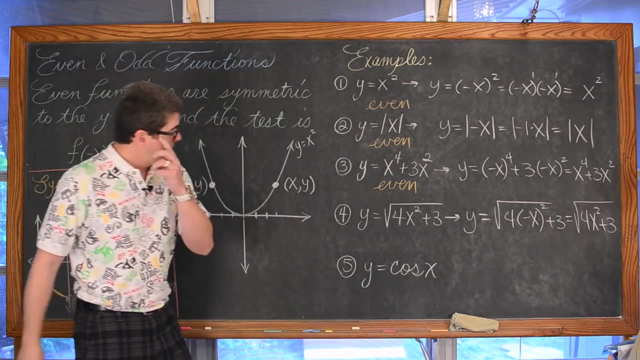 power is going to cancel out that negative, giving us an equivalent expression or the same expression back of the square root of four x squared plus three, Okay, And thus we got, We plugged in the opposite of x and we got the same expression back. 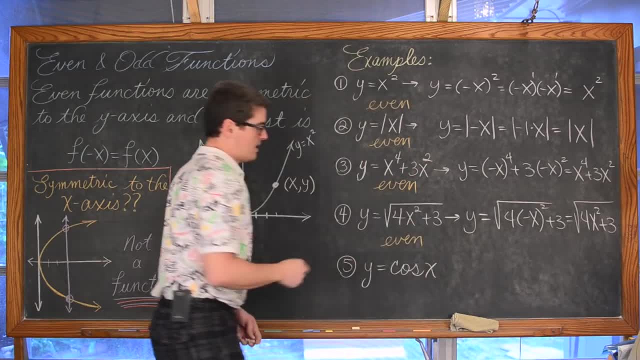 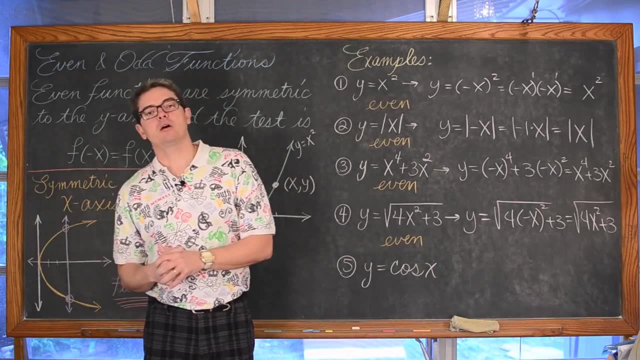 So this was even as well. Okay, Now for our last one here. I don't know if you have studied any trig yet or not. If you have, then you probably already know what the cosine graph looks like, and you already know that this is an even function. 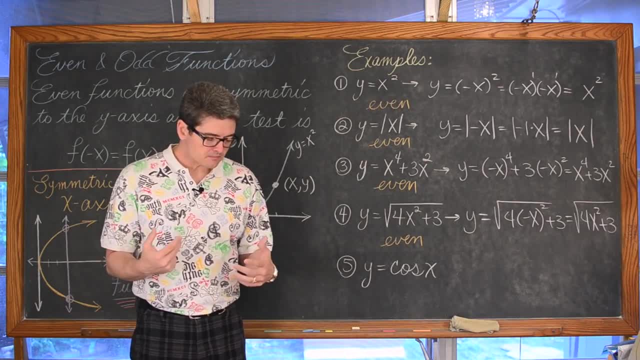 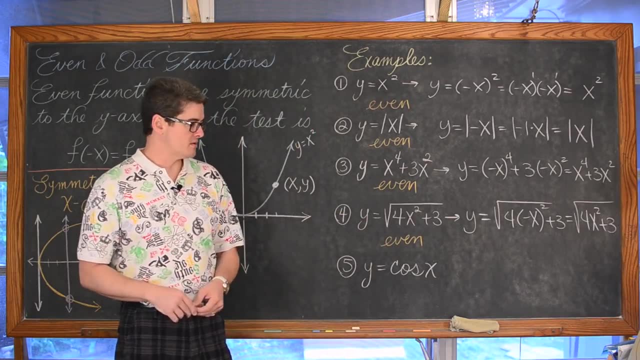 If you have not taken trig yet but you are allowed to use your calculator, then I would just basically suggest with this kind of question here I am kind of stuck with just testing some points And don't do just one. but you know, try the cosine of well, you are probably working. 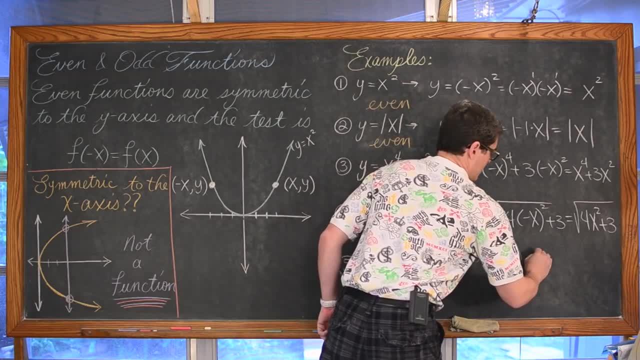 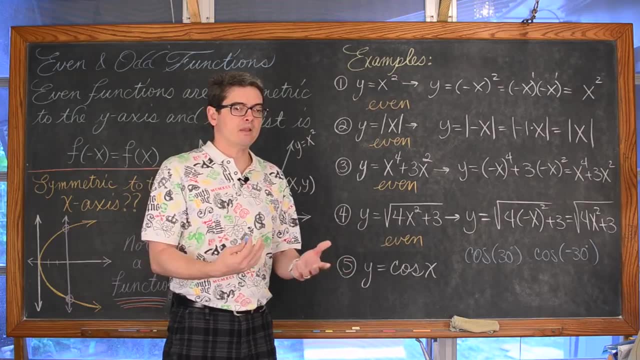 in degrees. so try the cosine of thirty degrees and the cosine of negative thirty degrees and see if you get the same answer. And by the way, now I know what is called a unit circle. again, I am not sure if you have studied that yet. 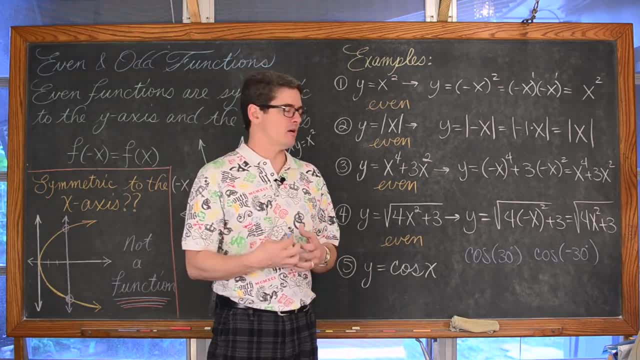 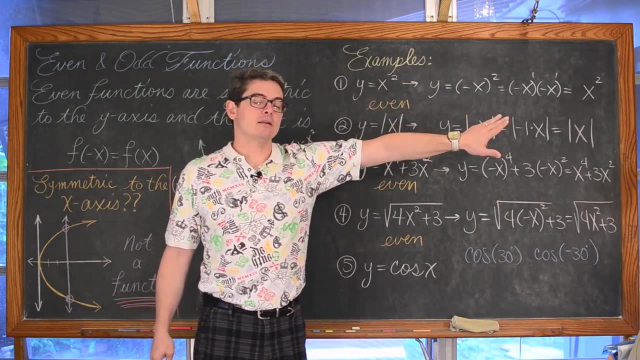 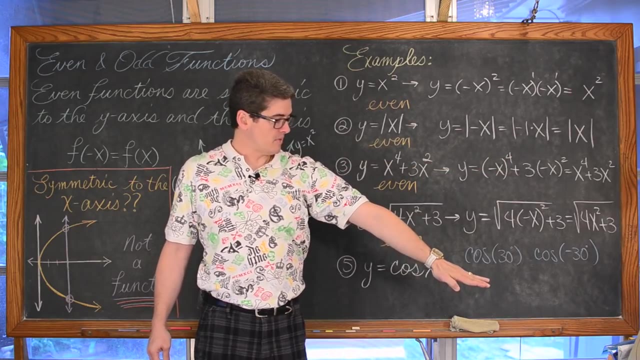 So I know what the exact value answer is. I am not sure what the decimal approximation is. So the cosine of thirty positive rotations are counterclockwise from the positive side of the x axis and negative thirty is negative. thirty Negative rotation is in a clockwise rotation from the positive side of the x axis. 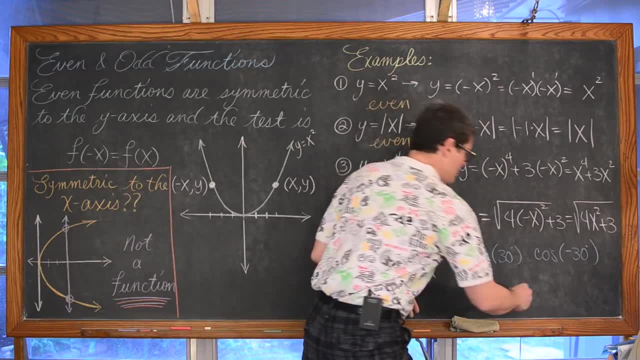 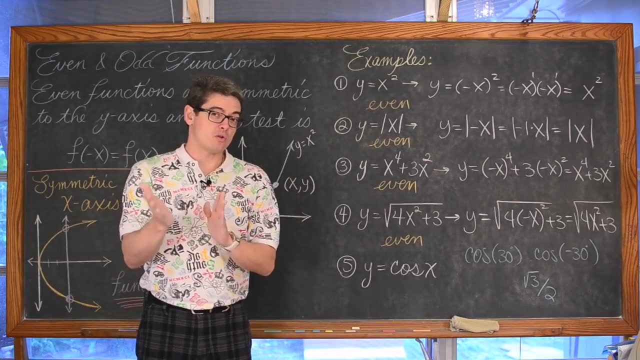 So the cosine of thirty and the cosine of negative thirty, that is going to be the square root of three over two. again, whatever decimal approximation your calculator gives you, as long as it is in degree mode, And if you try the cosine of thirty and negative thirty, the cosine of forty-five and the negative, 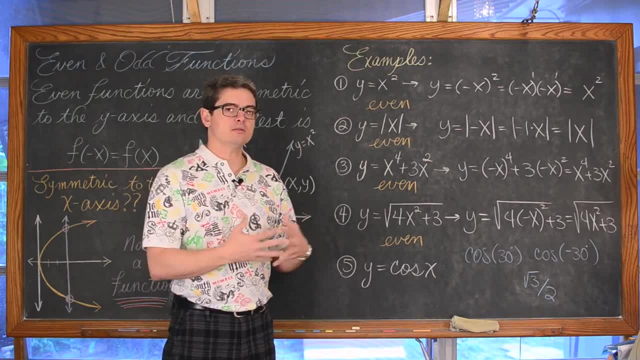 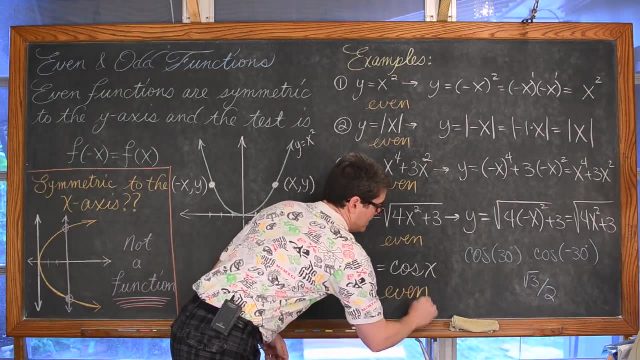 forty-five, the cosine of sixty and negative sixty. you are going to continue to get the same answer over and, over and over again, And thus the cosine function is an even function as well. Okay, so that is about all I can talk about for even functions. 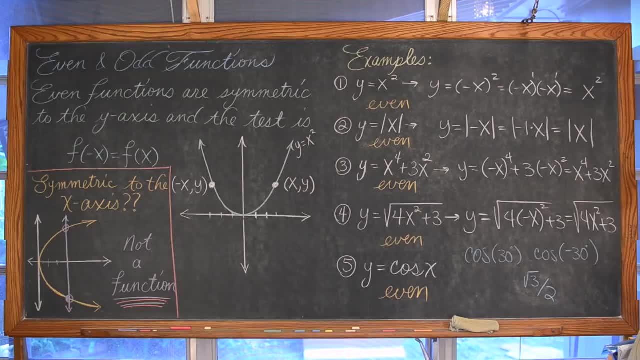 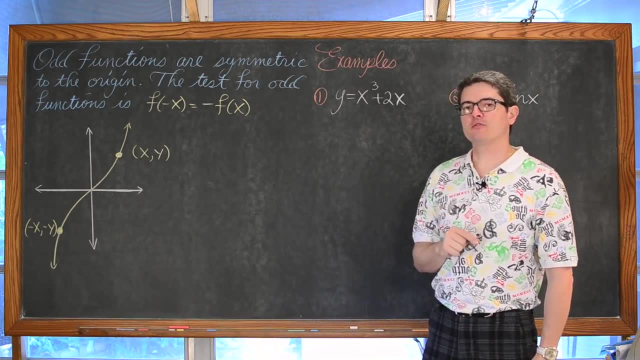 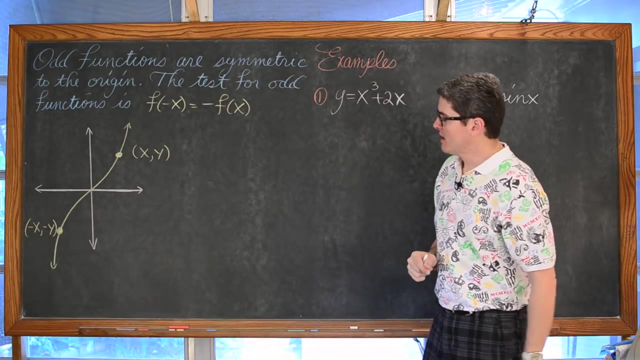 Let's get on to the odd ones. No, no, no, no, no, no Odd functions. Well, they are symmetric to the origin, and the test for odd functions is that when you plug in opposite values, You get the opposite answer. 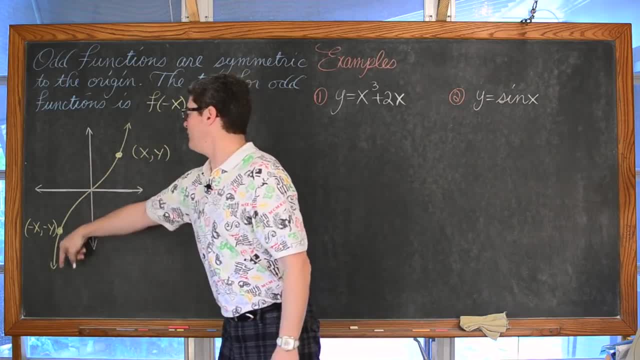 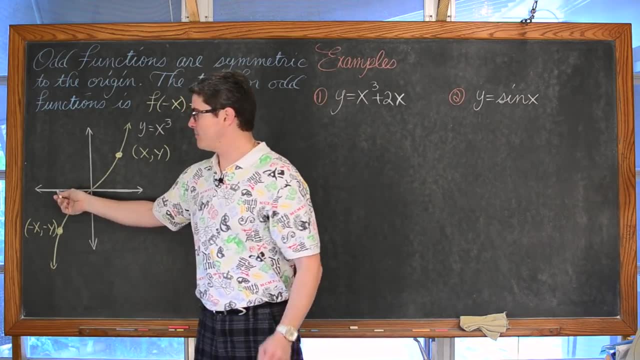 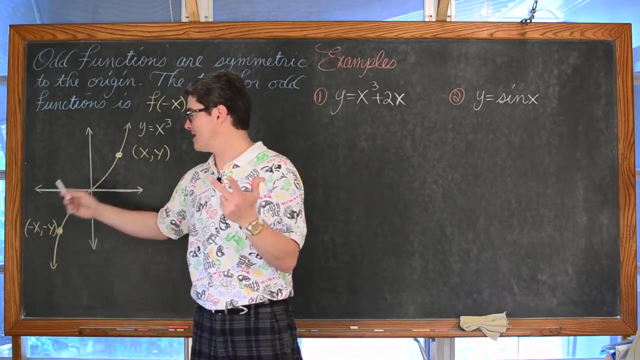 So we have an equation here. well, I have a graph and let's just say that is the equation. of y is equal to x cubed. Well, if you say, put in negative two, negative two to the third power, negative two times negative two is positive four times negative two is negative eight. 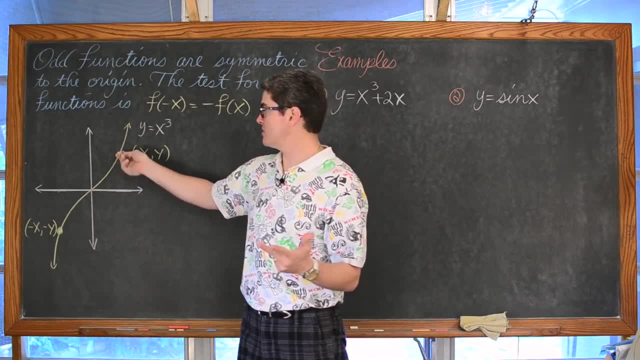 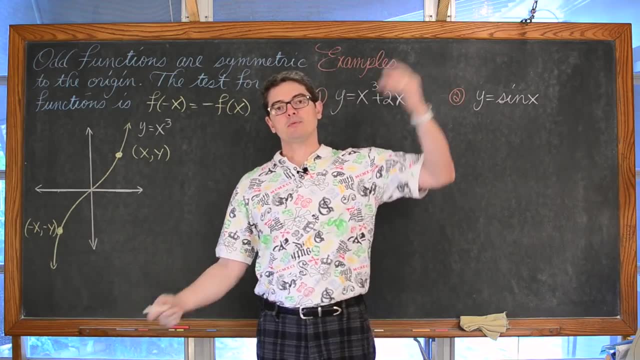 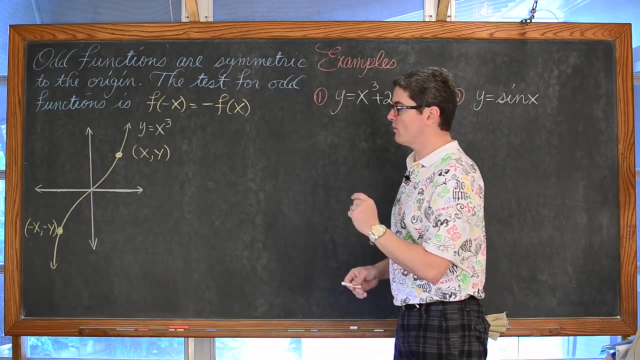 And if you plug in positive two, two times two is four times two is eight. So I have plugged in two opposite numbers, Negative two and positive two, and got out opposite answers, And so that is an example, graphically, of what your function may look like or will look. 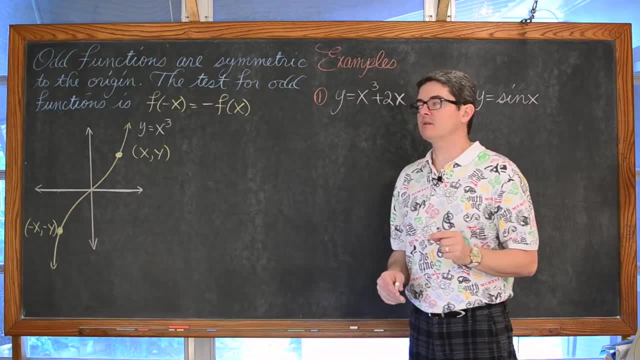 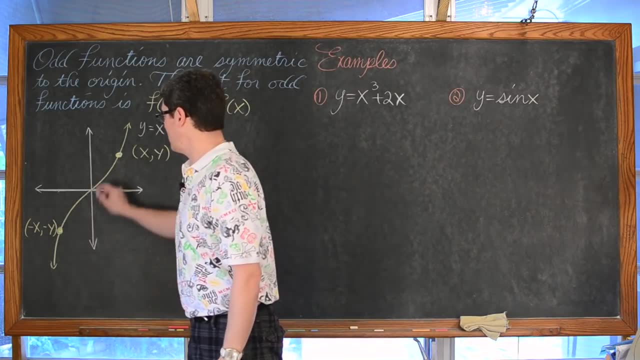 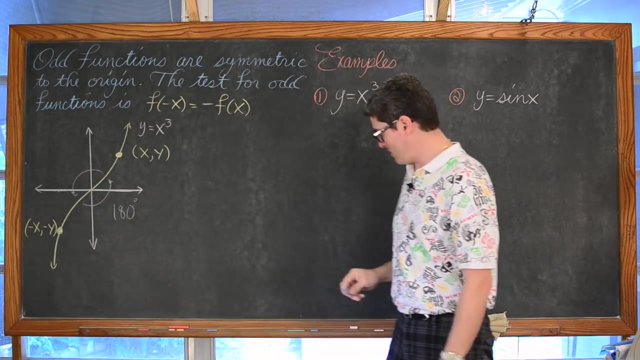 like if it is odd. Now we say that odd functions are symmetric to the origin. You can think of this in two different ways. You can see it as a rotation of a hundred and eighty degrees of rotation about the origin, Or Or. 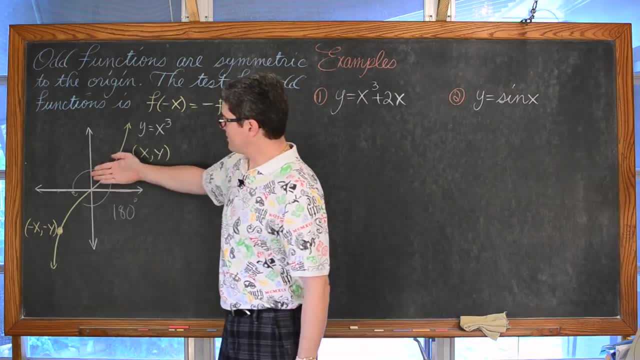 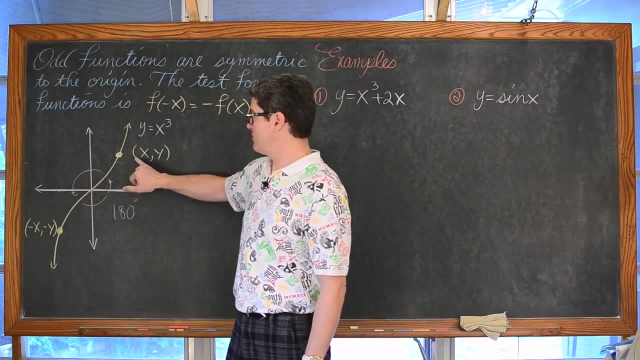 You can think of it as two reflections, where we take this portion of the graph and we reflect it over the x axis, which is going to give you- you know that would be, we kind of talked about that already- symmetry to the x axis, even though it is not really a function. 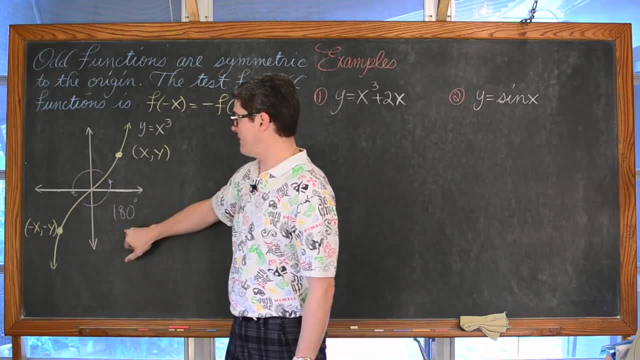 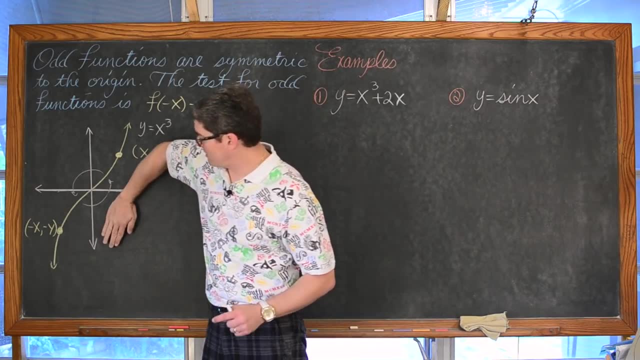 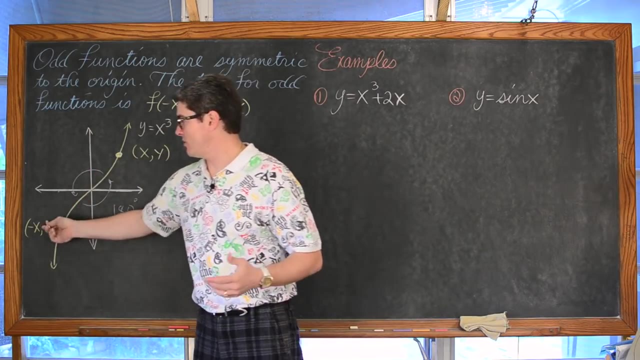 Where you would have the same x value but getting the opposite y value. So if you reflected this point over the x axis, you would be down here at x negative y. And then you do a second reflection Where you take that and you reflect it over the y axis and you end up with your opposite. 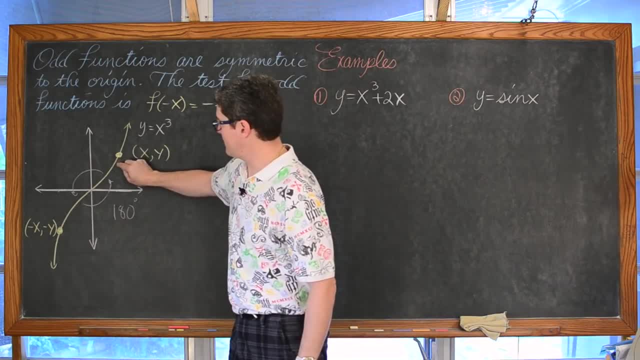 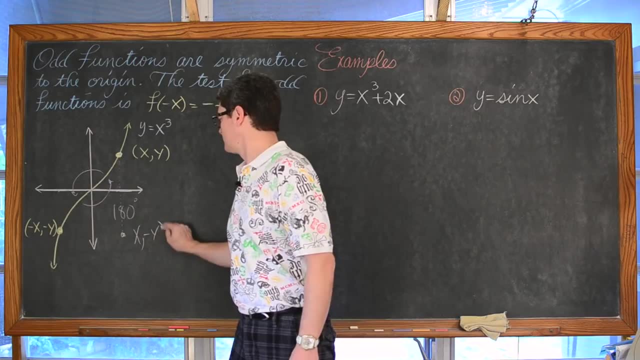 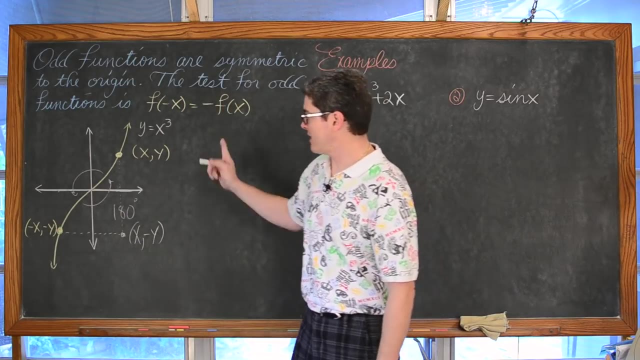 x, opposite y, or negative x, negative y. So you can think of it again as two reflections, One reflection being over the x axis And then a second reflection taking that over the y axis, finally landing you at the point negative x, negative y. 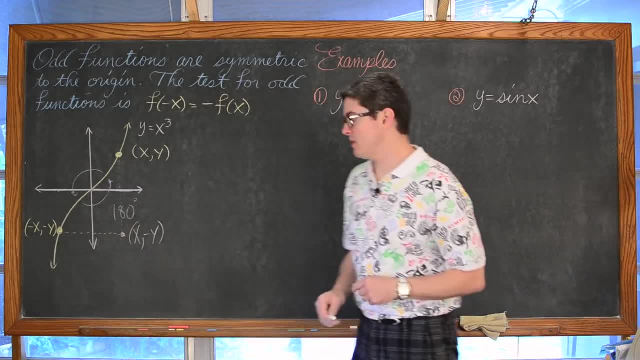 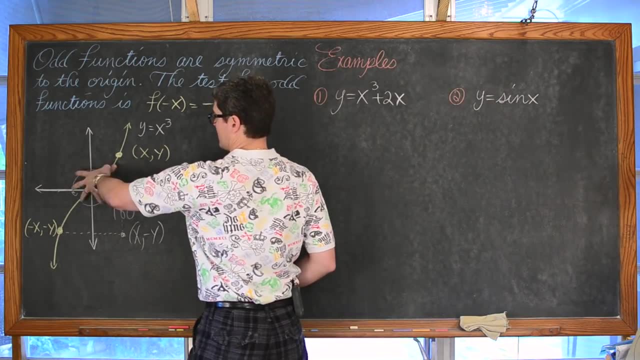 Because when you reflect over the y axis, Like we talked about in the previous screen, you will change the sign of the x coordinate. Ok, I like to focus on the fact that you can take this and rotate it 180 degrees and have the 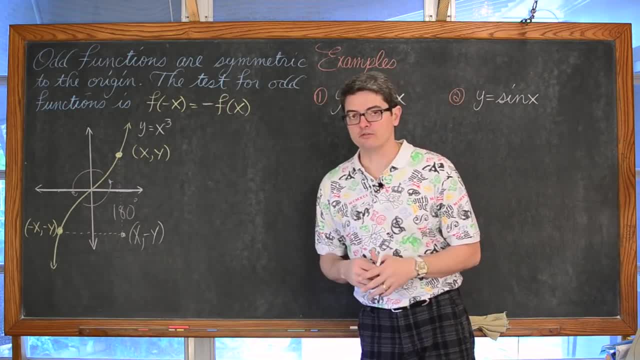 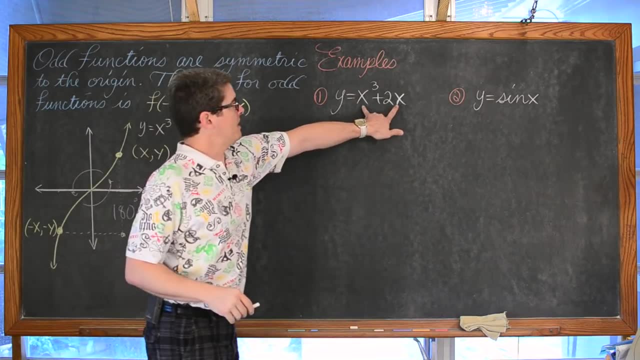 graph perfectly line up on itself, But there are times where you want to see those two reflections as well. So our two examples- actually there is going to be more than two, but the ones that are on the board right now. We have again just a basic polynomial. 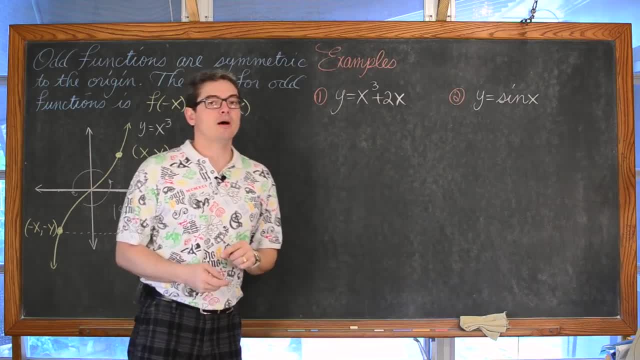 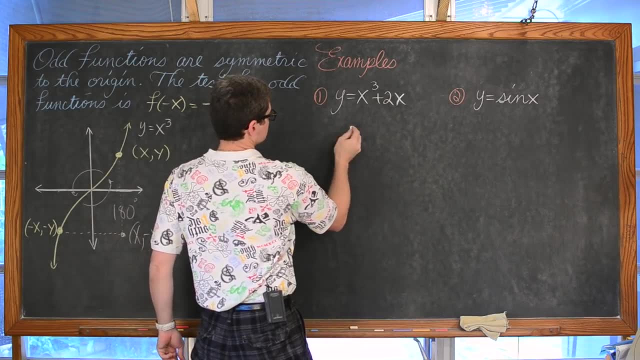 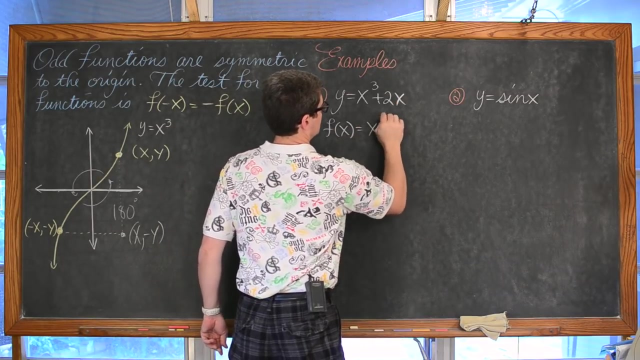 We have one independent variable and all of those exponents are positive integers And When we plug in the opposite- Ok, The opposite of x- Let me go ahead and this time write this as function notation, Just to give you a different look there. 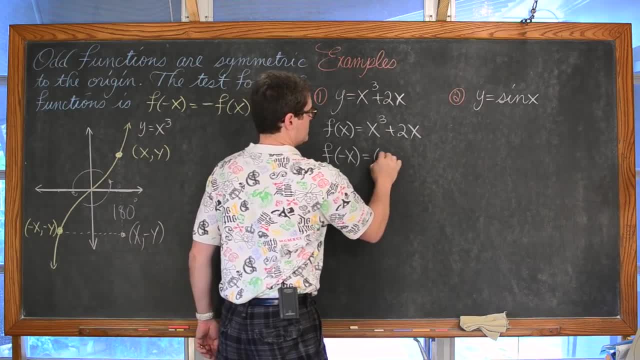 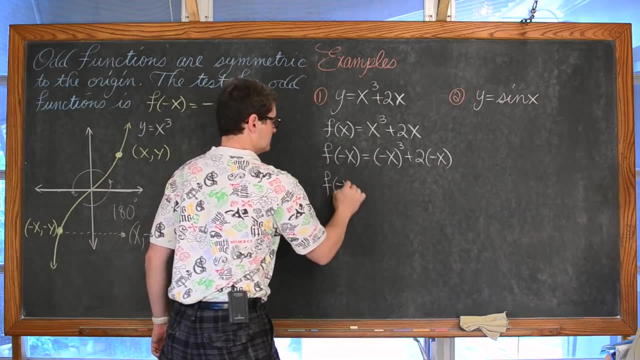 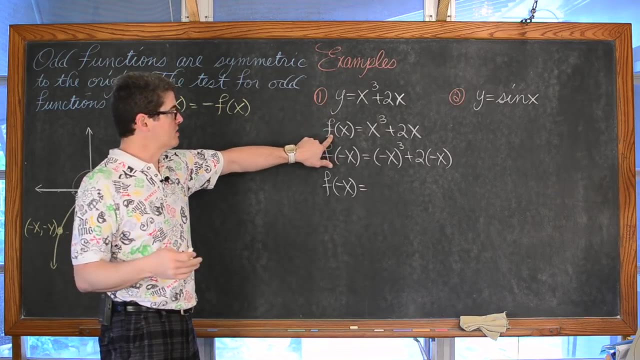 And we have f of negative x is equal to negative x cubed plus two times negative x, And you know function notation It. There are lots of times in mathematics when we are dealing with more than one equation where we would like to have those equations named. 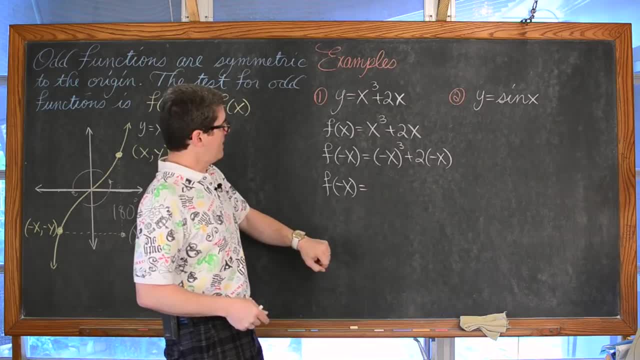 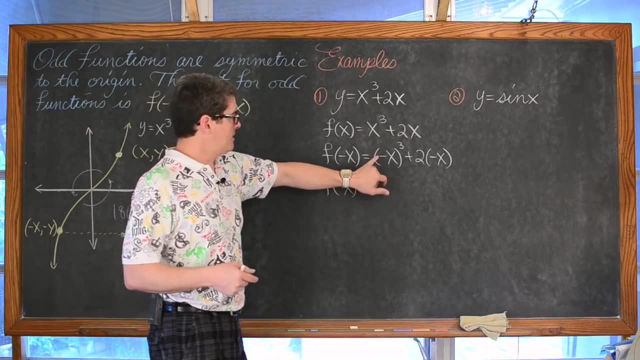 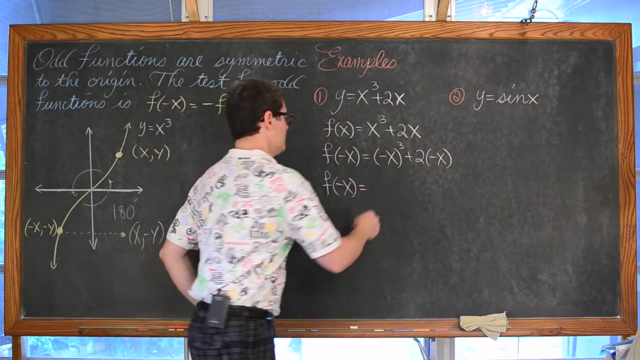 Those functions named. So that is now function f And just recognizing that that function notation, like in this case f of x is a replacement for y And negative times, itself negative, one times negative. one is positive, one times negative, one again is negative, x cubed. 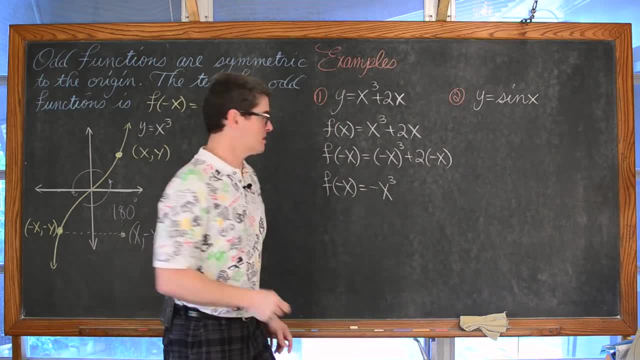 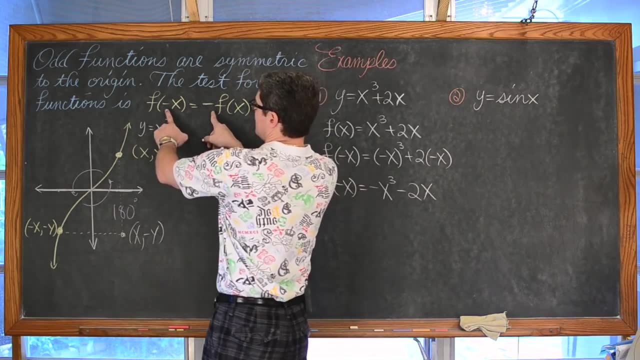 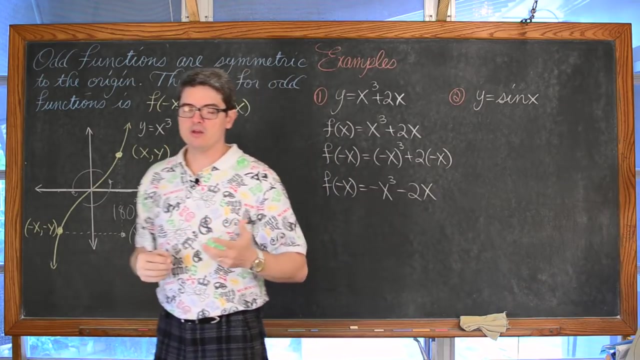 And negative, Or positive, two times negative one. So negative. two times negative one is going to be negative, two x. Ok. now this notation here, this function notation, opposite numbers in opposite numbers out. Well, with multiplication you can create an opposite number by simply multiplying by negative. 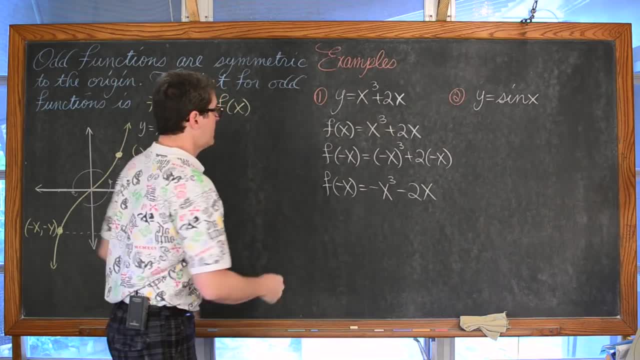 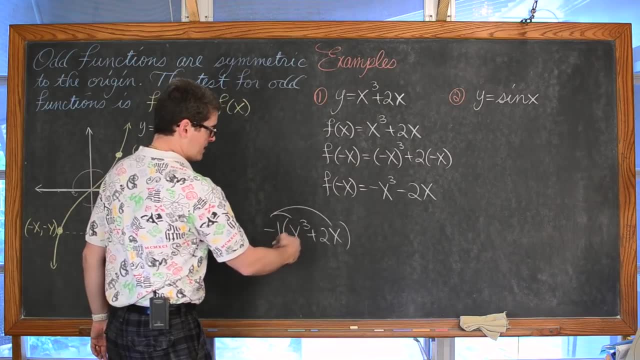 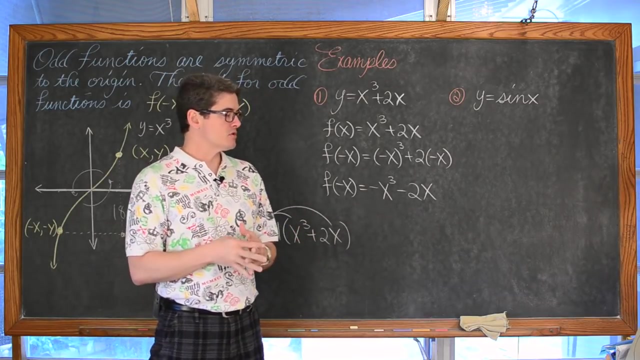 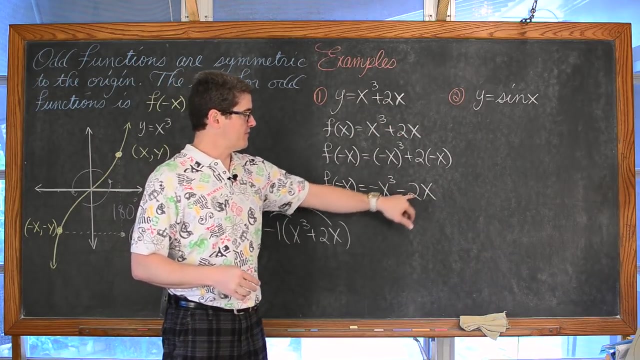 one. And if I take this equation and multiply through negative one, I would get Negative x cubed minus two x. So with polynomials- not true with all functions, but with polynomials- if you see all those signs change, every single sign of each of these terms. if they all change, then you: 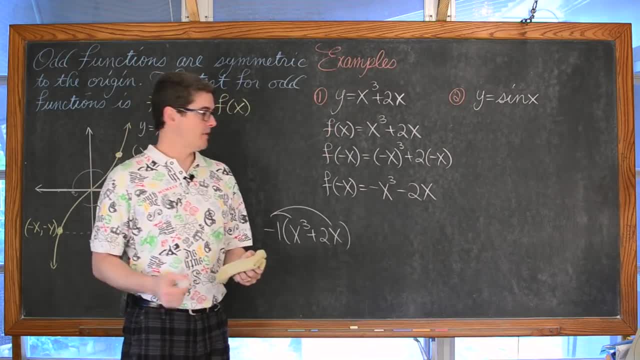 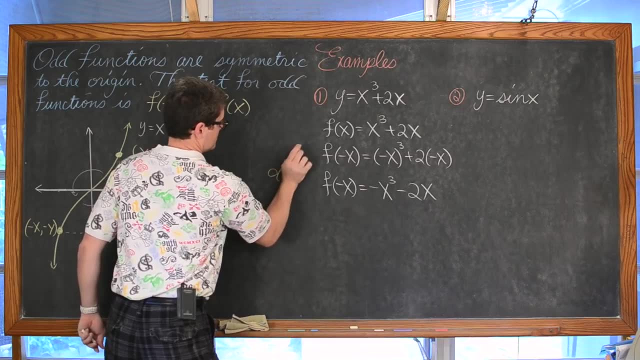 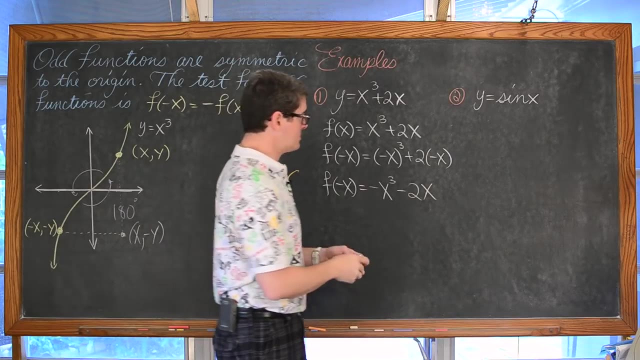 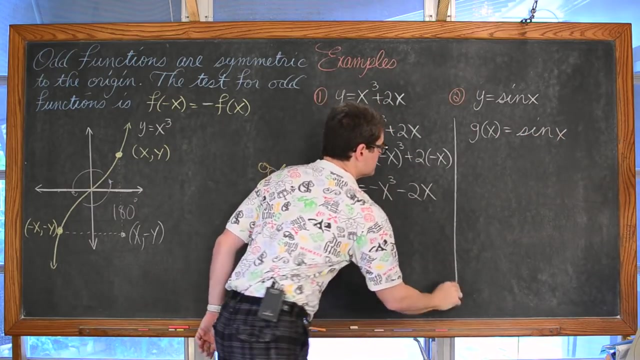 are looking at an opposite expression, And thus this is an odd. Where is my orange chalk at This is an odd function, Now, moving on. Moving on to y is equal to sine of x, or let's call this: g of x is equal to sine of. 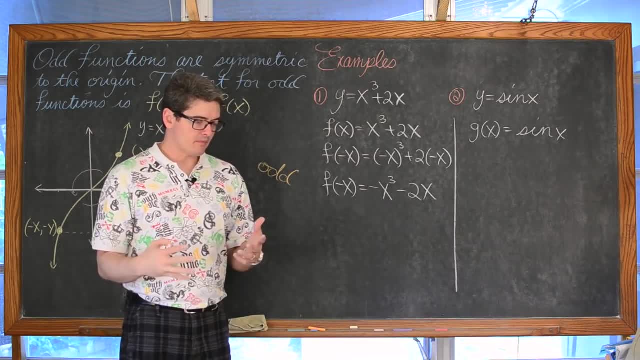 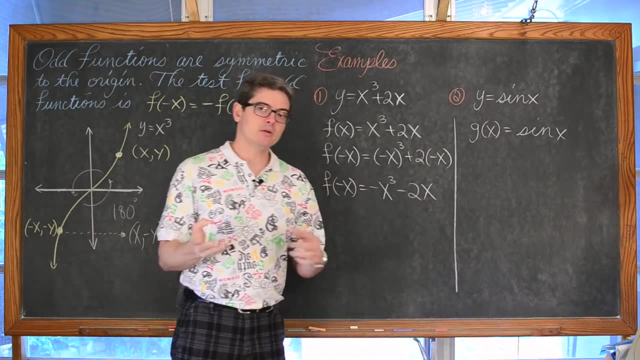 x. Again, if you are just starting on your journey of algebra, you haven't dealt with your trig functions yet. you might want to just make sure your calculator is in degree mode and test a few values with your calculator. If you know the unit circle, use that. 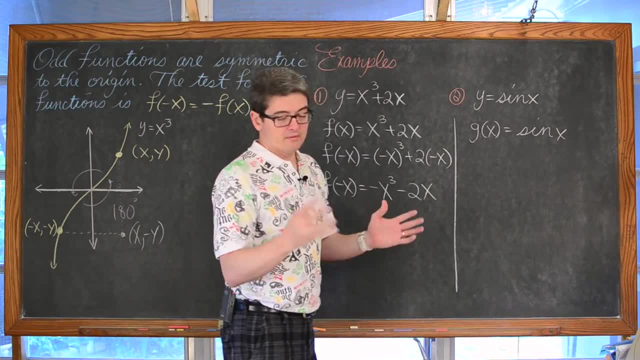 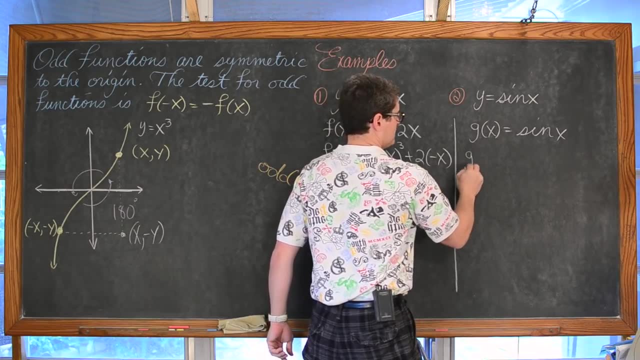 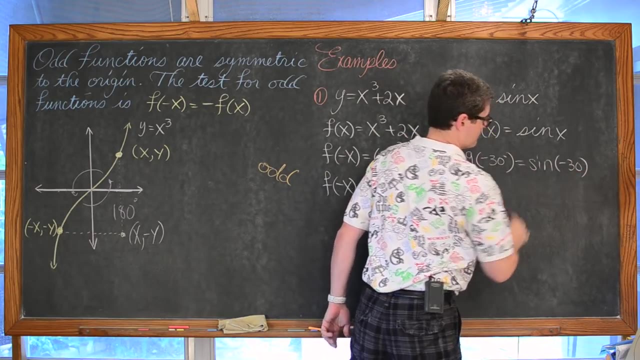 If you know the graph of these trig functions well, then you are set And you are probably already on to the next question. So let's see what g of negative thirty degrees is. So that is going to be the sine of negative thirty. 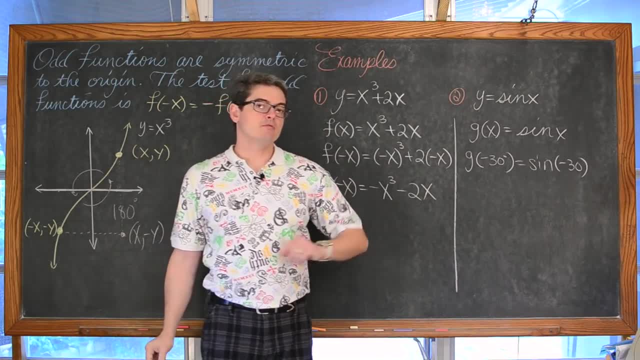 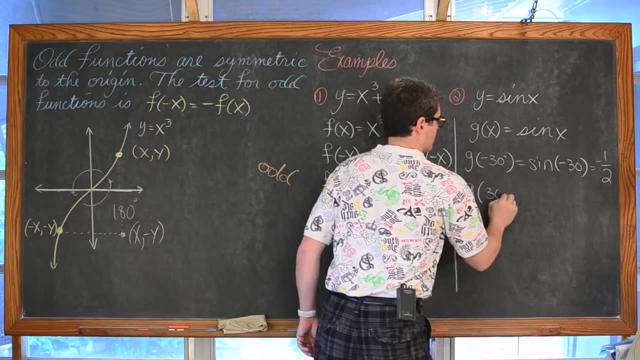 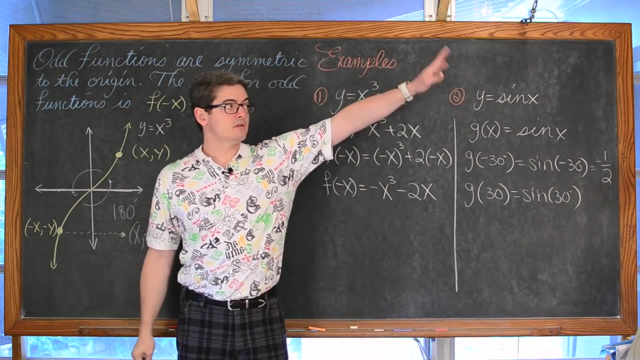 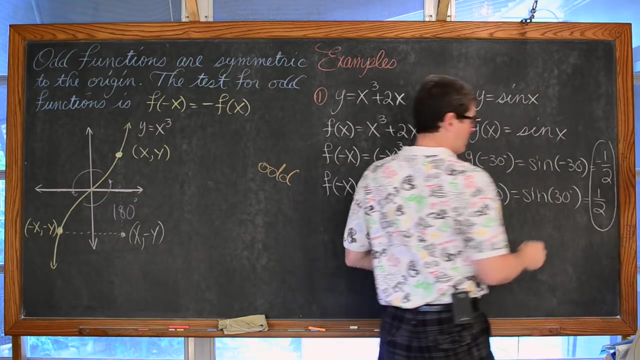 The sine of negative thirty degrees is going to be equal to negative point five or negative one-half, And g of positive thirty, as a sine of thirty degrees is going to give us positive one-half, And indeed we have Woo. That even hurt my ears. 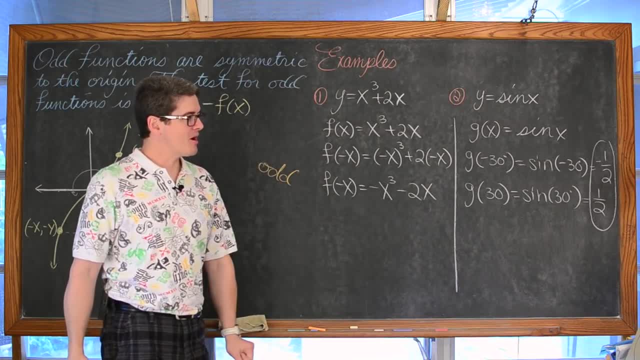 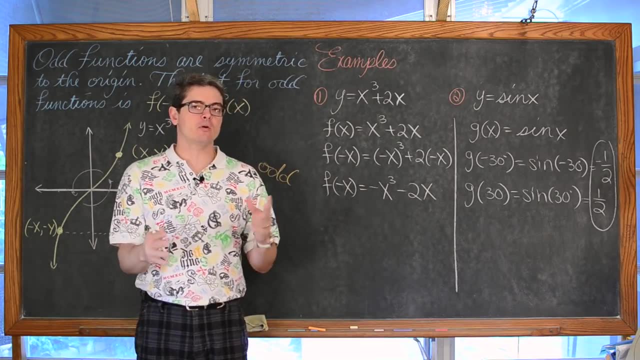 Sorry about that. if you are listening to on the headphones, We plugged in our opposite numbers and got opposite answers. So now one test point. you know, for a function to be even or odd, this symmetry has to exist for every single point in existence. 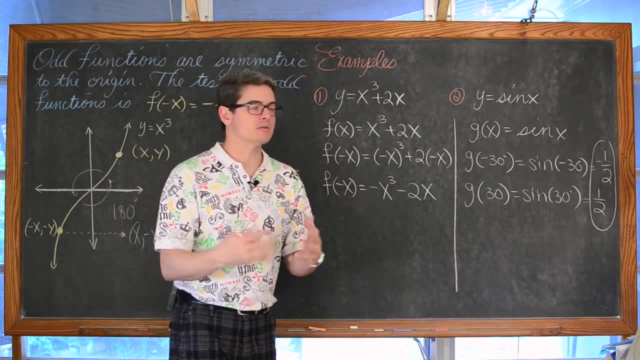 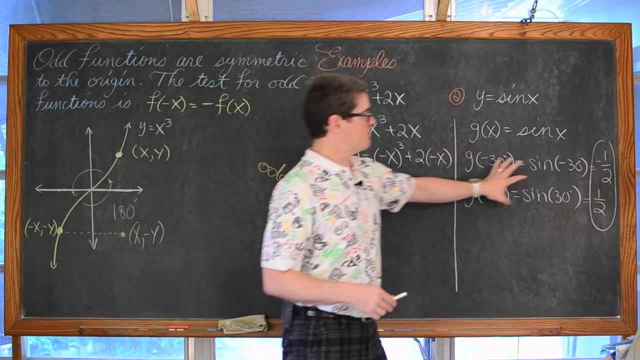 Like an infinite number of pairs of points, opposite points. So you might want to check this a couple, two, three times This. certainly We don't want to do a proof of you know, trying to show this in general, Probably not. 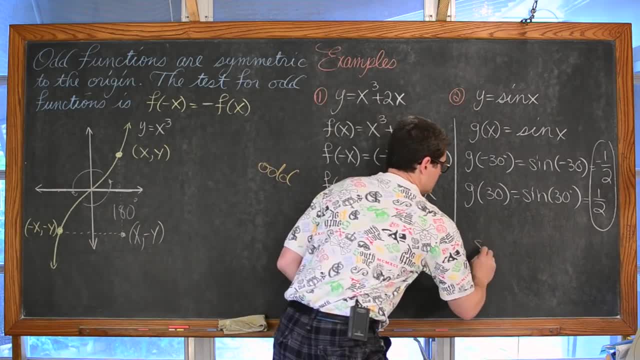 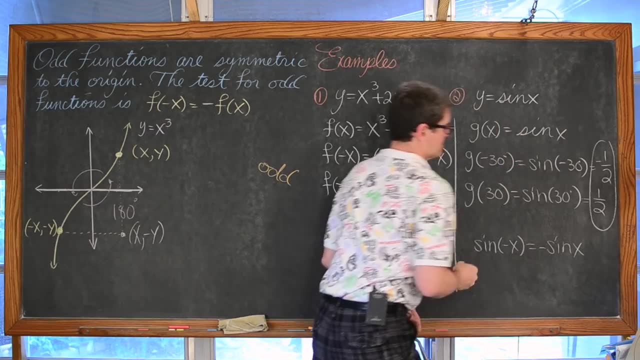 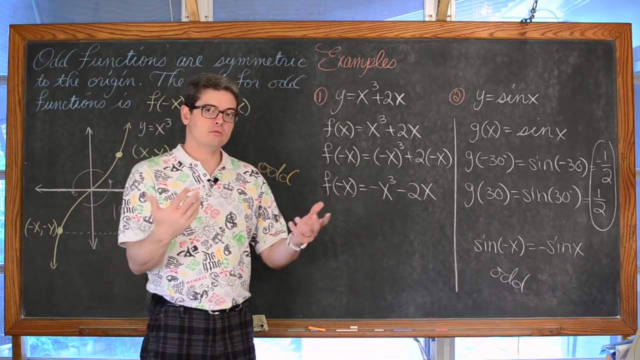 We don't want to use general terms, really, other than to say that the sine of negative x is equal to the negative, or the opposite of the sine of x. This does indeed come out to be an odd function as well. I would suggest that you again test more than just one point or a pair of opposite. 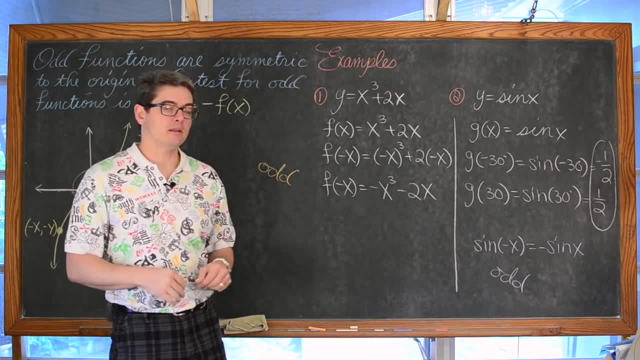 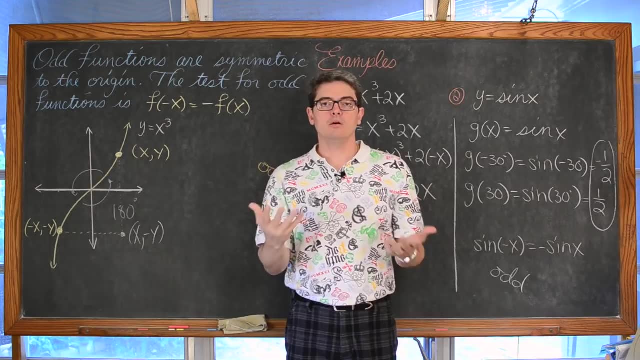 numbers before you come to that conclusion. And then, if you have a graphing calculator, grab that as well and make sure that graphically it does look like. you can take the calculator and turn it upside down And see, you know the same that it appears to be, the graph is lining up on itself. 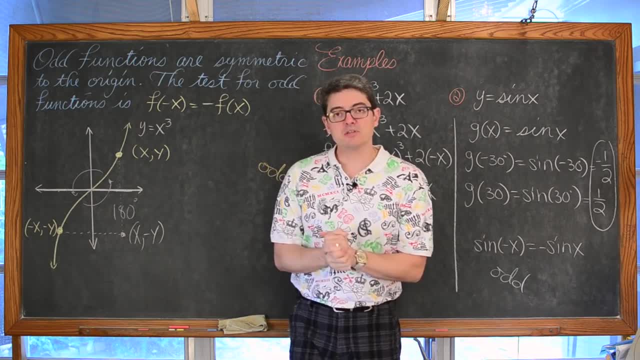 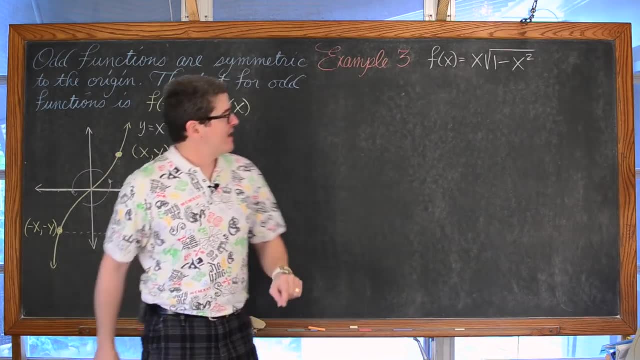 You get the same picture. Okay, so we got a couple more examples. Let's get to those right now. Bam, No, no, no, no, no. For our third example we have: f of x is equal to x times the square root of one minus x. 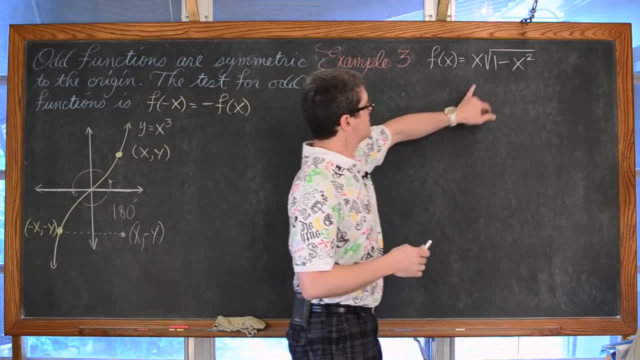 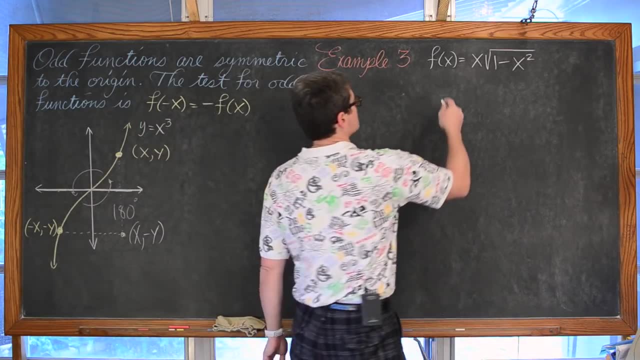 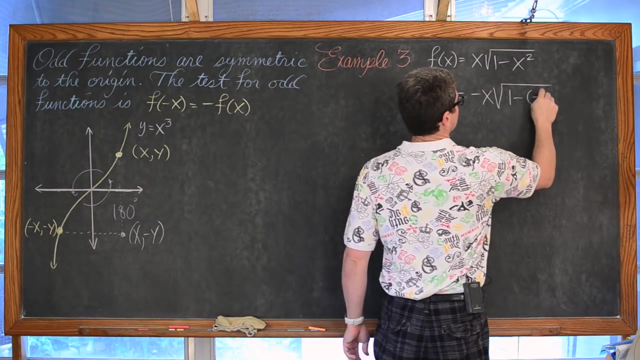 squared? Certainly not because of the radical in here. We don't have a basic polynomial function. Let's go ahead and plug in the opposite of x and see what happens. So we have f of negative x is equal to negative x times the square root of one, minus the opposite. 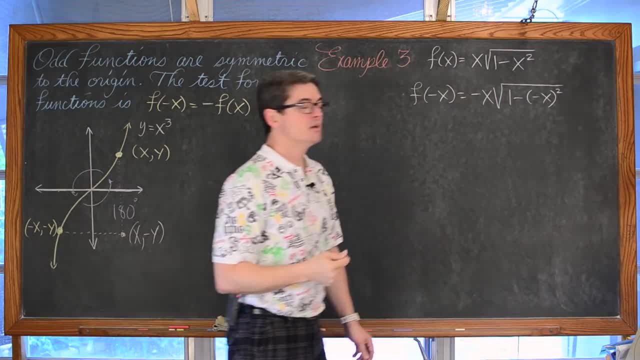 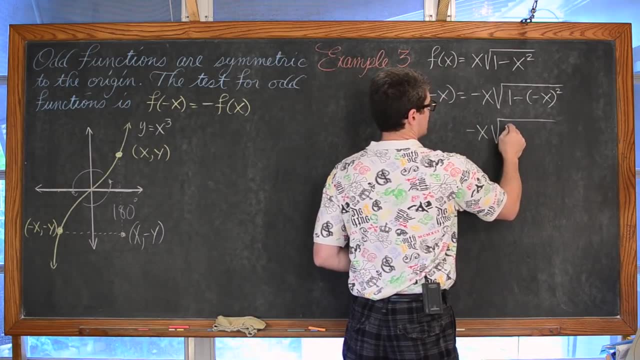 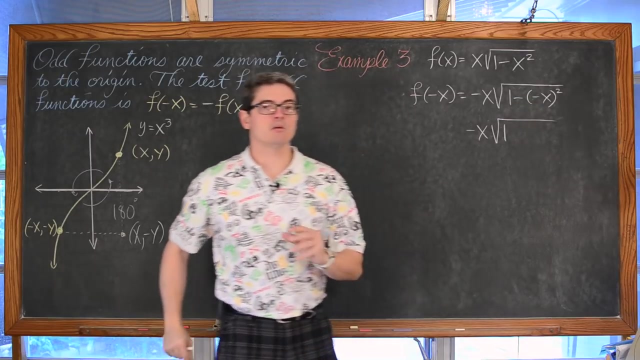 of x or negative x. we should say the opposite of x squared, keeping that in parenthesis, And we get negative x or the opposite of x times the square root of one. okay, so one what? Because you know we see that we have two negatives here. are we going to let those? 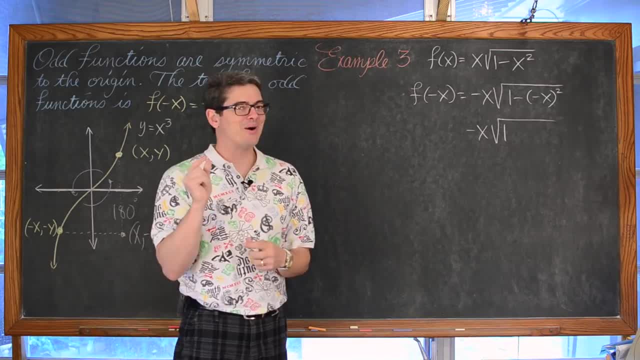 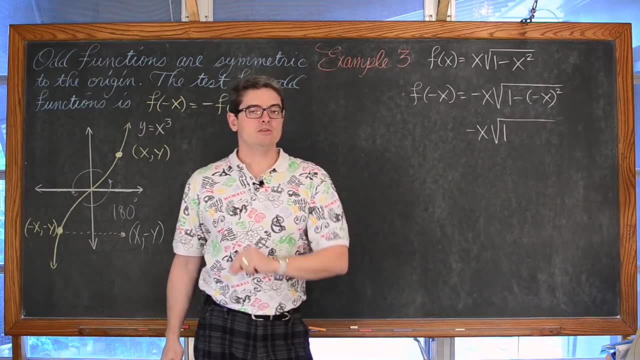 two negatives cancel and create a positive, Or Or are we going to correctly apply the power of two? first See, if you let these two negatives, just you know, hit each other, see that they are side by side and go, oh, that's positive. well then you're doing multiplication before you apply. 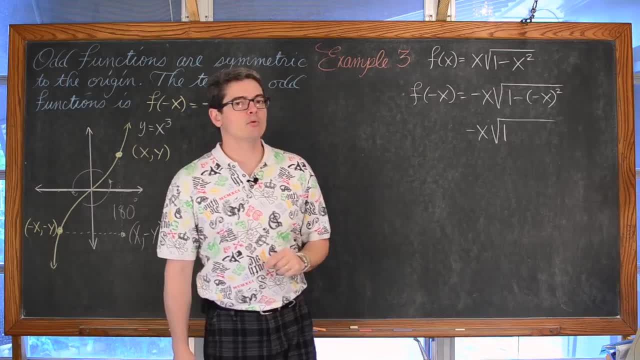 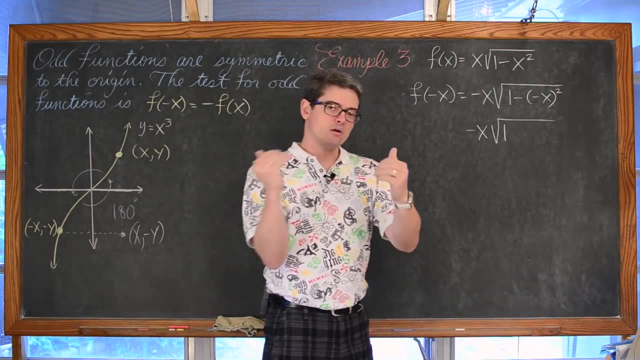 an exponent, And that does not follow, of course, the PEMDAS, the order of operations, Please excuse my dear Aunt Sally. parenthesis: exponents, multiplication and division, You know, those are on equal plane, whatever comes first, left to right, and then finally, 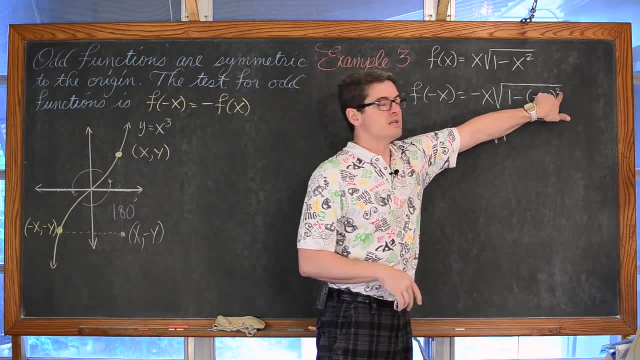 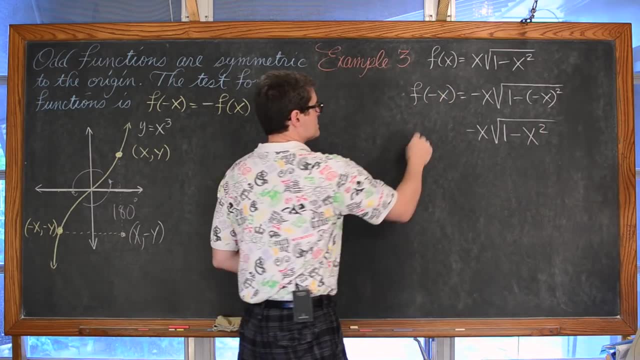 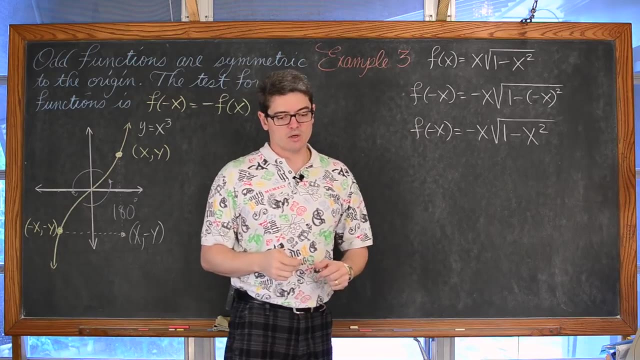 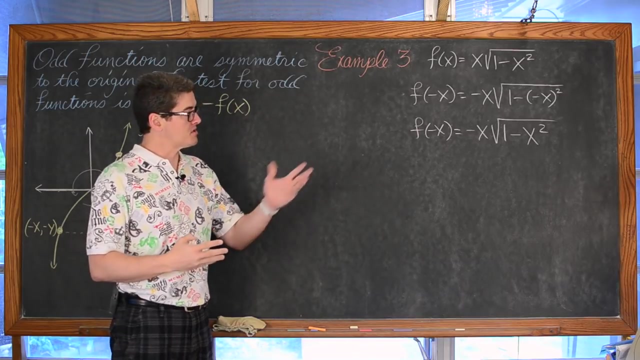 addition and subtraction. So negative one times negative. one is positive. Okay, Negative one is positive one. so this is going to be one minus x squared. Now let's look at how this equation compares to the original one. You know, all the signs didn't change, so maybe it's not odd. 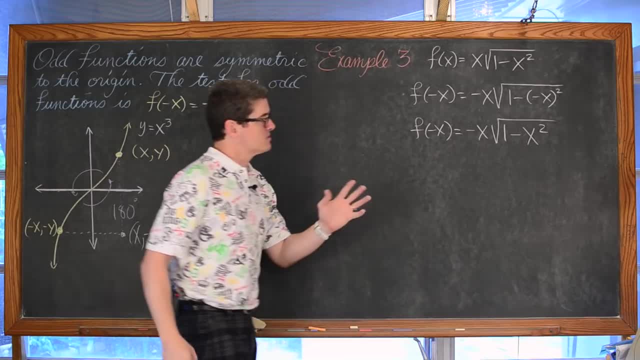 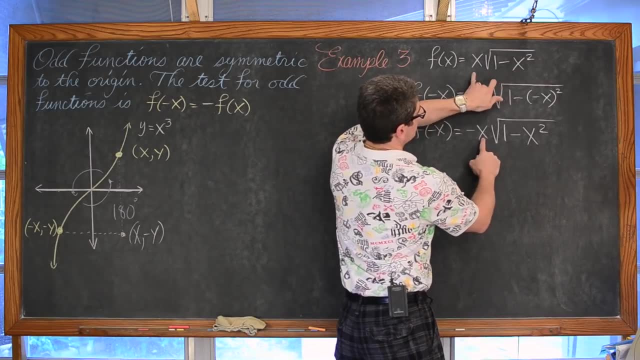 It's certainly not the exact same equation, so it's not even so, is it neither? Well, again, follow in the order of operations: When you take a number and you plug it in for x. and if I look at these two expressions, 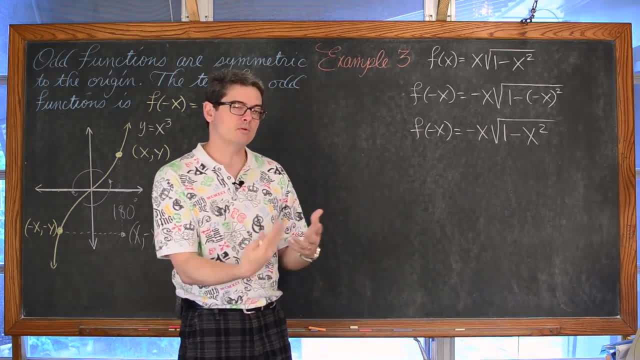 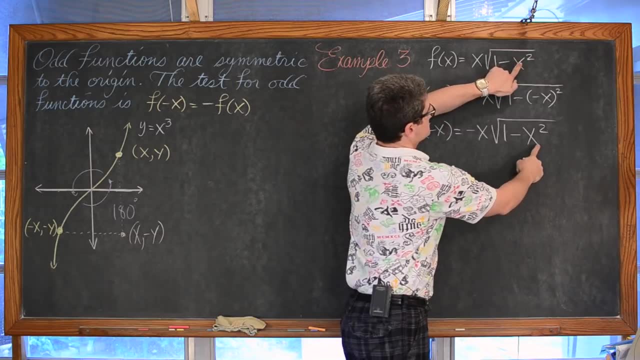 and I see that they both have the same variable and I'm evaluating them at the same time. I'm going to be assuming, of course, that whatever x is represented is the same for both of these expressions. So something is getting squared, that same something is getting squared and it's one. 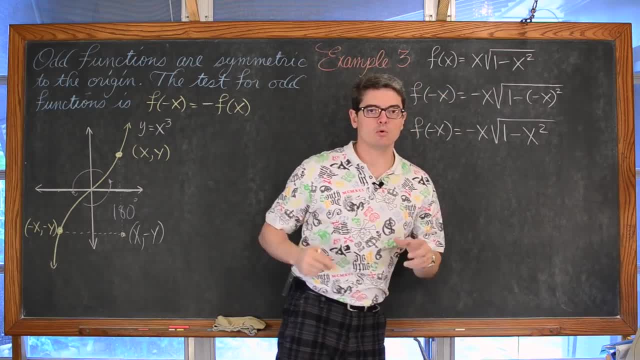 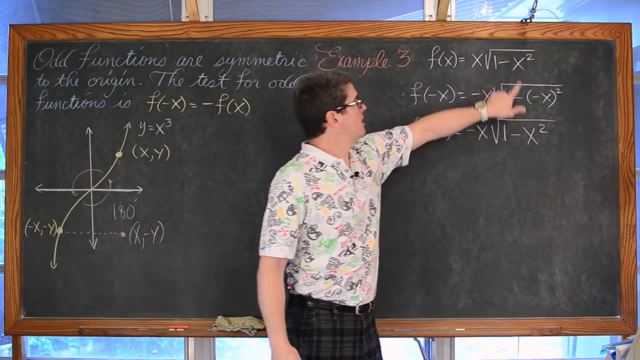 minus that same something. So the expressions inside the square root symbol, where you have to start working first, are the same And then working your way out of the grouping, The grouping symbol, the square root symbol. we're going to have the square root of one. 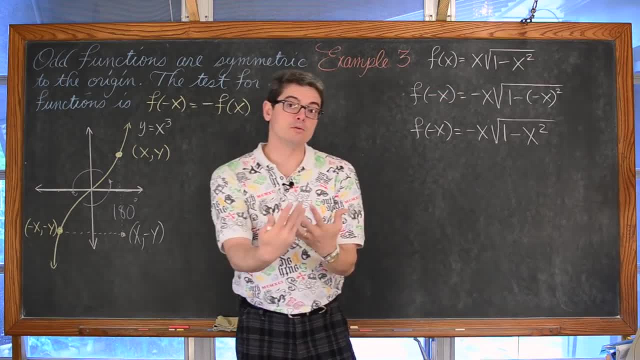 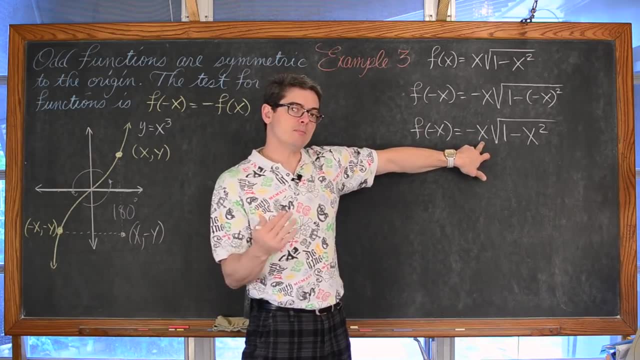 minus x squared, the square root of one minus x squared. so they're equal so far. And then, finally, whatever this answer is is getting multiplied by x, and whatever this answer is is getting multiplied by the same number but with a different sign. 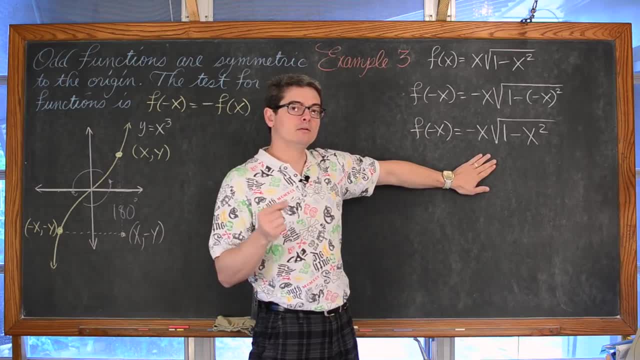 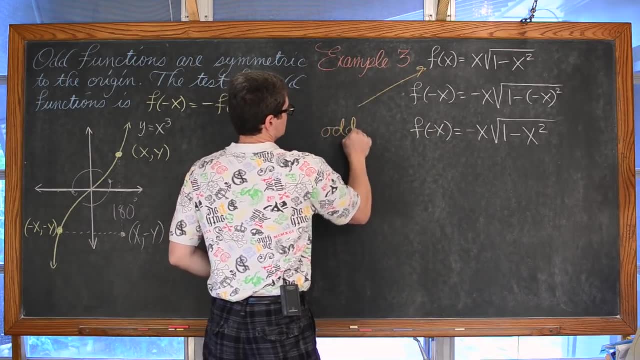 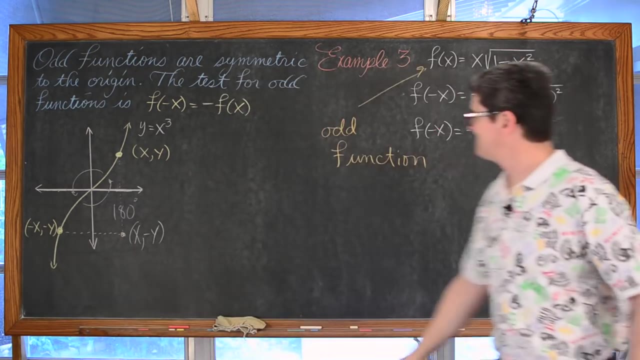 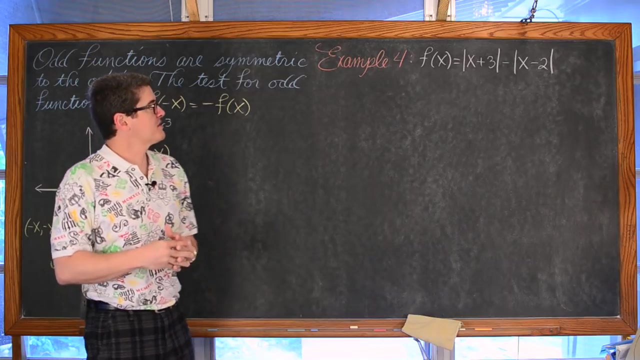 So actually these are going to be what Opposite answers. So this is A non-function. Next example, Example number four for identifying non-functions, We have: f of x is equal to the absolute value of x plus three, minus the absolute value of. 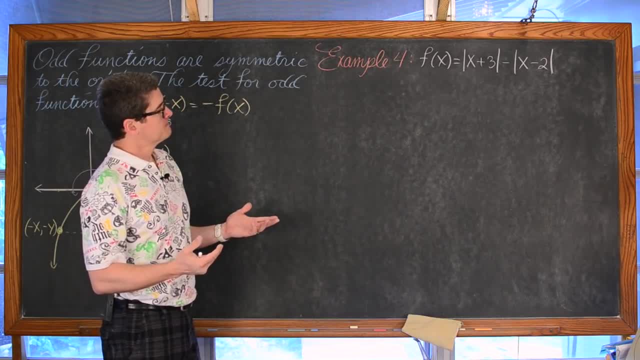 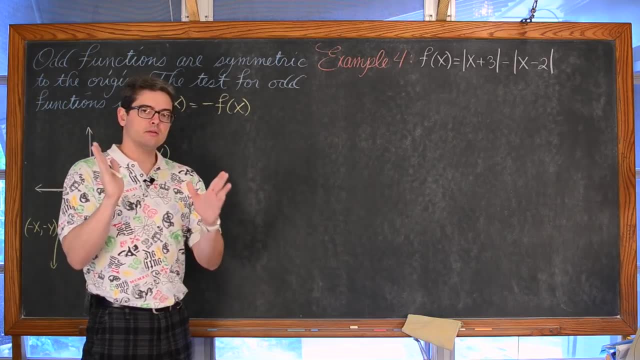 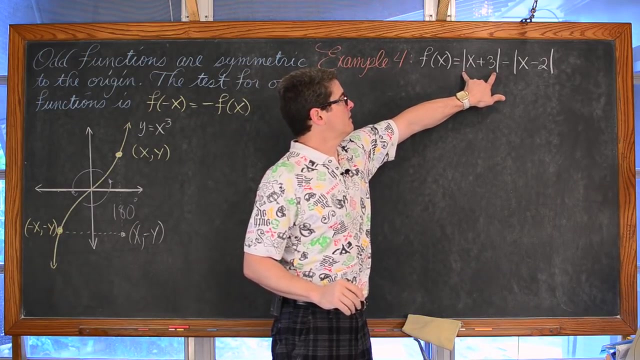 x minus two. Again, the absolute value functions are a little bit tricky. They're not just basic grouping symbols And again, these absolute value graphs will always have a sharp bend somewhere And something is special happening with that placement of that sharp bend, with these absolute 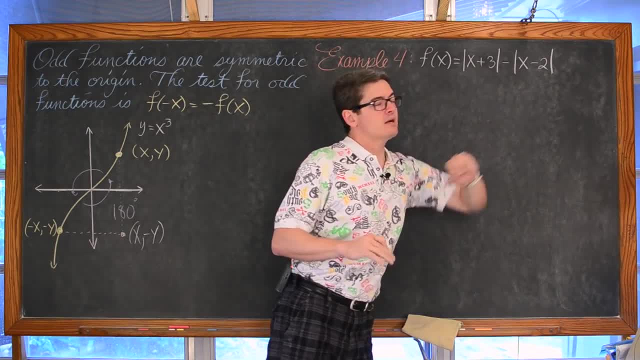 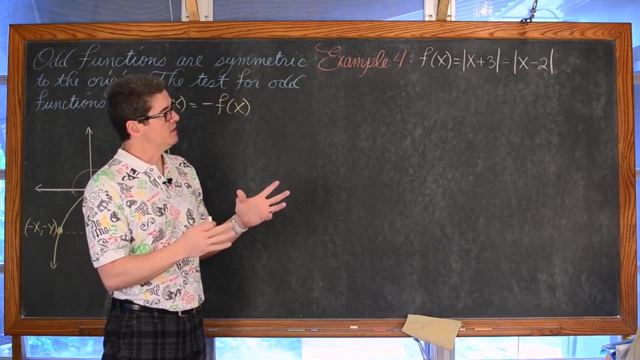 value functions are going to occur where the inside expression equals zero, But not thinking about that for at the moment and going okay. well, I know that these are sort of a bit more complicated than many of the other types of functions that we deal with. 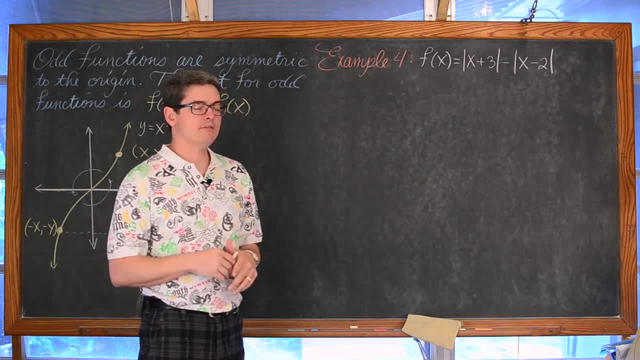 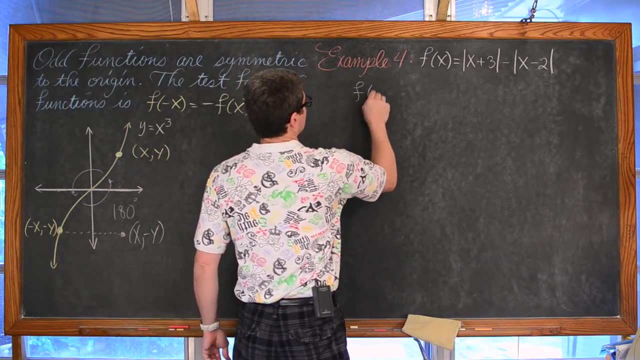 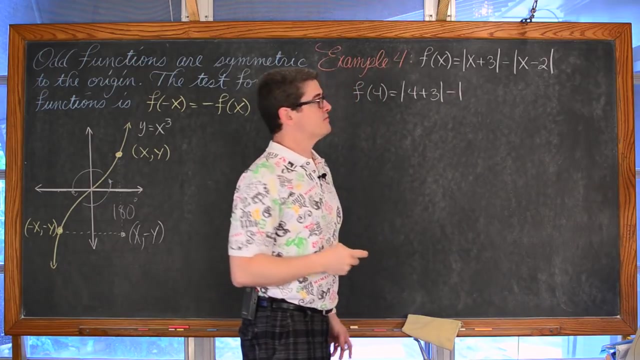 I don't have a graphing utility to simply graph this to see if we have any symmetry to the origin. So I'm just going to plot some points, I'm just going to test some points, some opposite values. Well, f of four is equal to the absolute value of four plus three minus the absolute value. 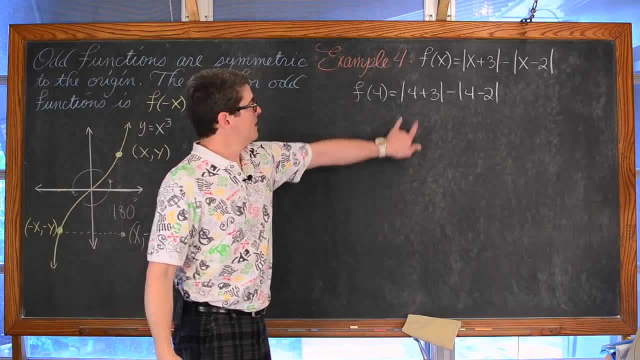 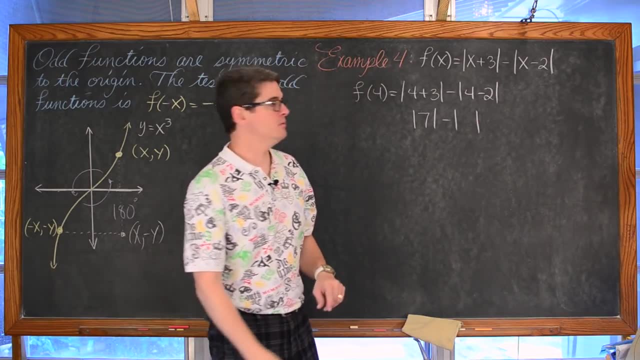 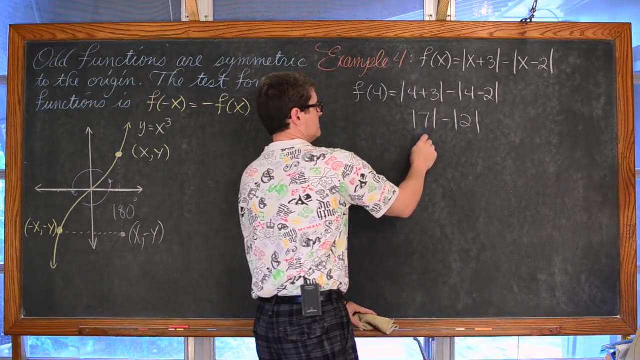 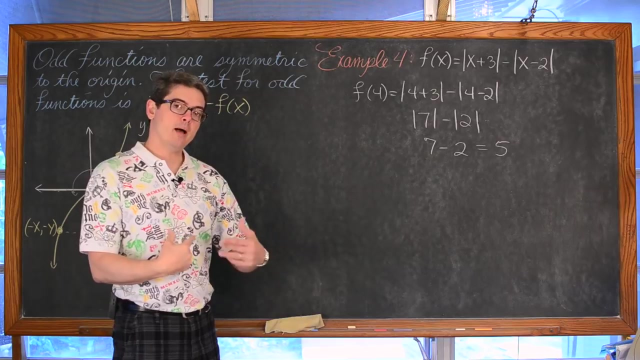 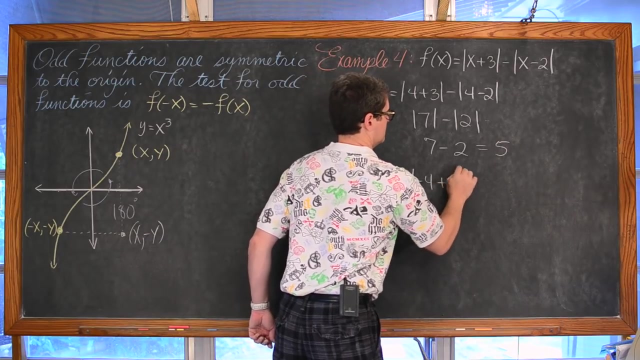 of four minus two, And that's going to be the absolute value of seven minus the absolute value of two. And Well, Probably shouldn't be skipping steps. Seven minus two is equal to five. Alright, Well, let's try plugging in the opposite of four. 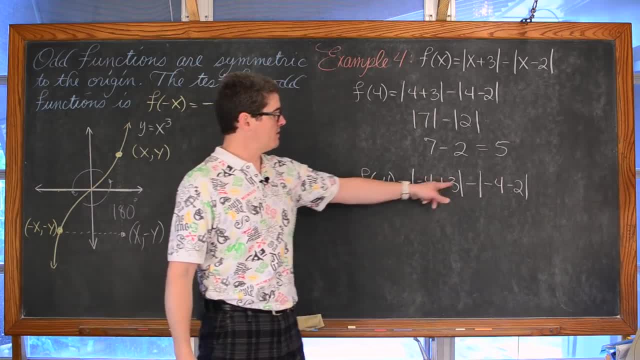 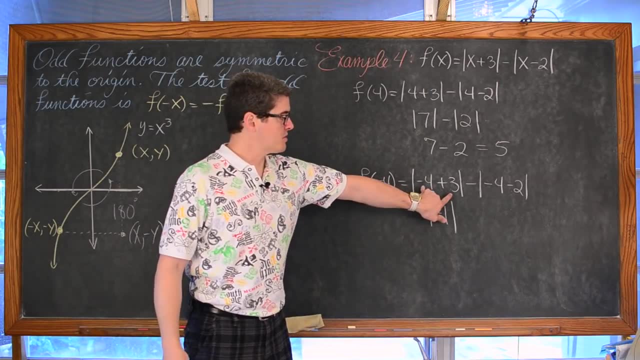 When I plug in the opposite of four, which is negative four, we get the absolute value of negative. four plus three is the absolute value of negative one. Uh, Again, there's two terms in here, so I'm not going to drop both of these negative signs. 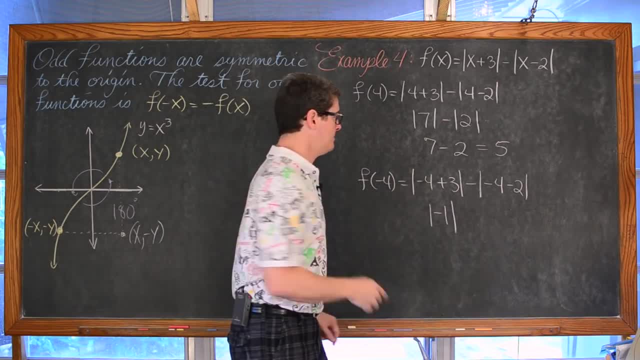 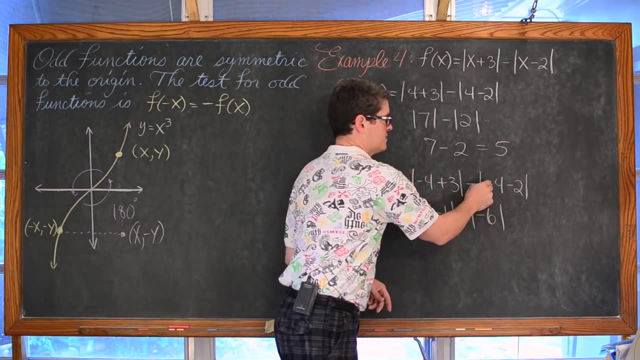 and say that it's four plus three is seven. That is an incorrect statement. When you combine two numbers, well, assuming you're not multiplying. when you add two negative numbers or combining two numbers that both have the same sign, you want to add those. 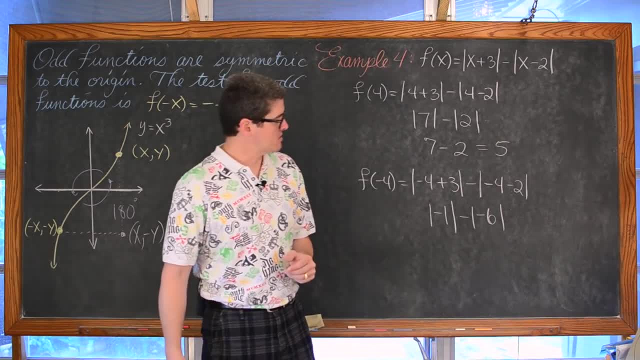 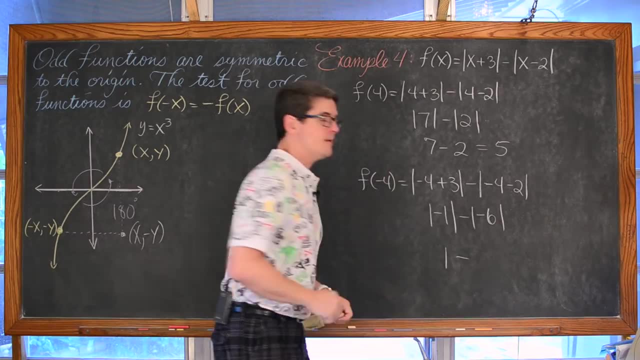 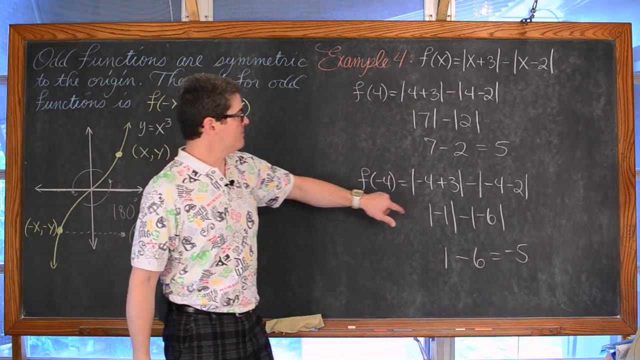 numbers and keep the sign. So negative four minus two is going to be equal to negative six And the absolute value of negative one is one. The absolute value of negative six is six And we get an answer of negative five. So we plugged in opposite numbers and we got opposite answers. 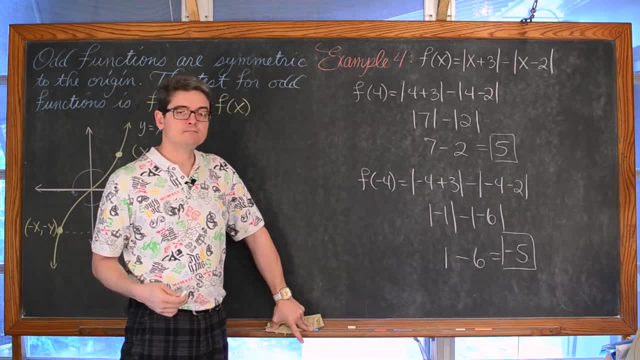 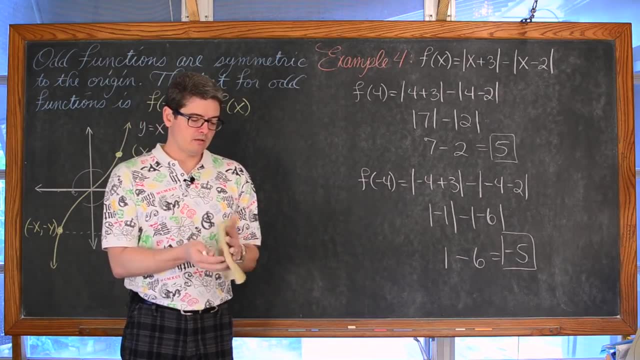 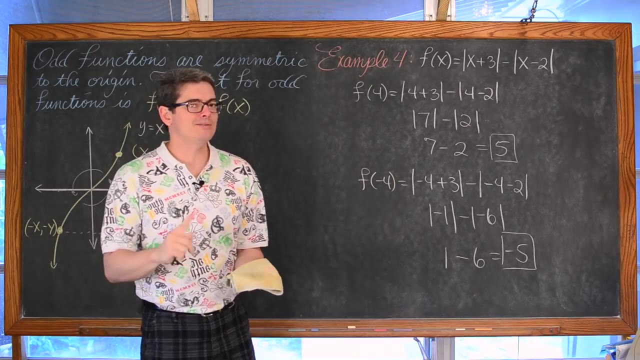 So this looks like it's an odd function. Great, It's not. That's why you need to test more than a couple of points when, if you can't work out the problem in general, pure algebraic terms, In your testing points, you can't do just one pair of opposite numbers. 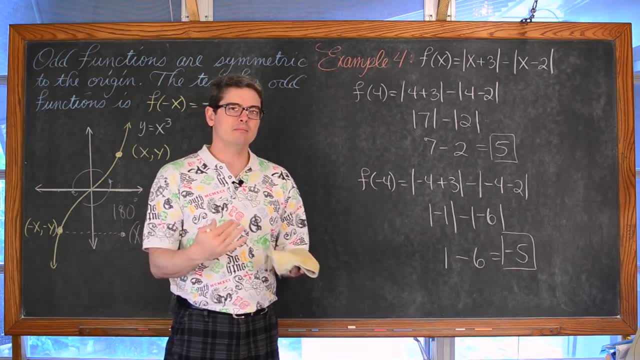 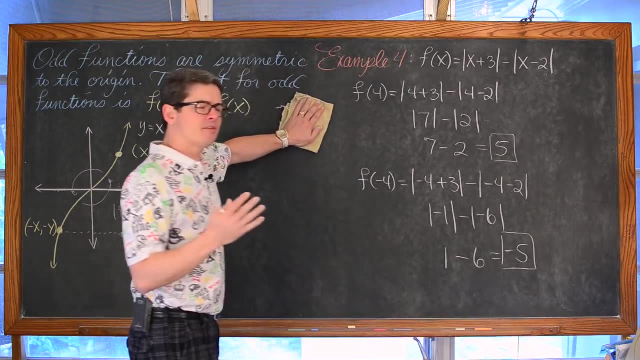 You need to do multiple sets to kind of make be more sure of your answer again, or use a graphing utility if you have it available, And also put a little bit of thought into it. Now. I mean, you know, maybe we put some thought into this, but if we're going to try another, 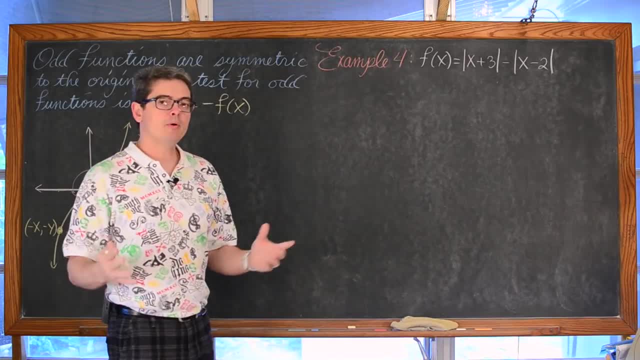 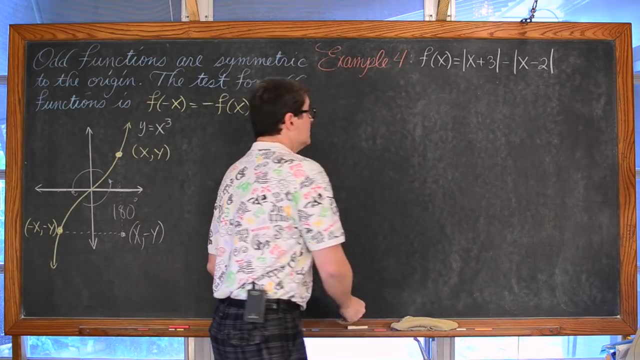 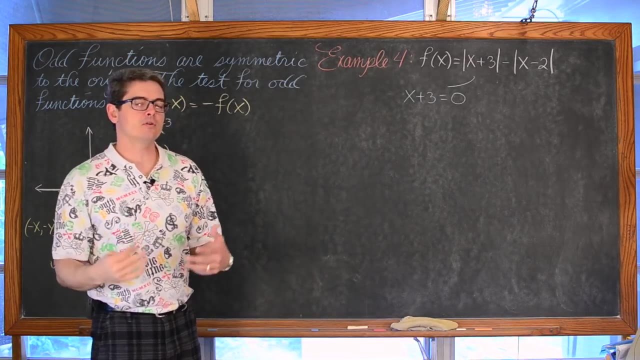 couple of numbers. I'm not going to just pick them willy nilly and just hope that. well, not hope, but just you know I guess. yeah, I hope I get the right answer. So this expression x plus three, the sharp bends for absolute value functions, occur when: 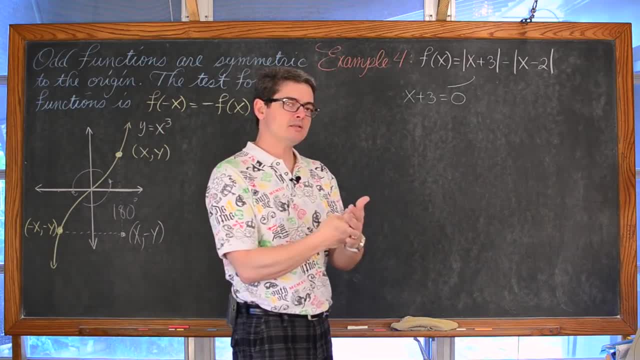 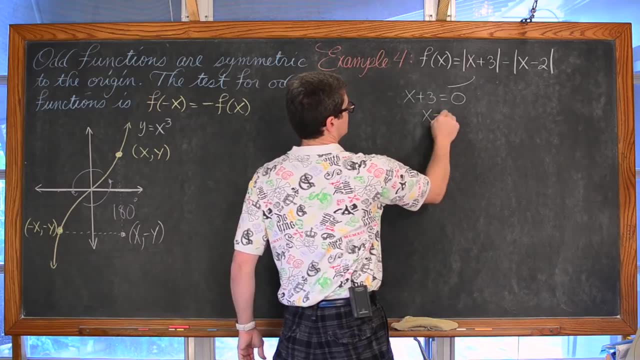 we can make the inside expression equal to zero. That x value that makes the inside equal to zero. that's where the sharp bend is going to be. Well, if I take that and I set the x plus three equal to zero when I subtract both, 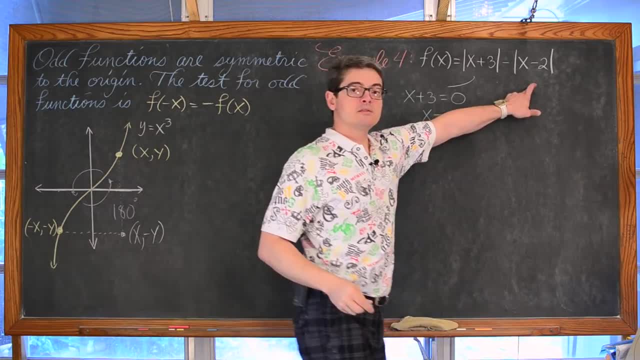 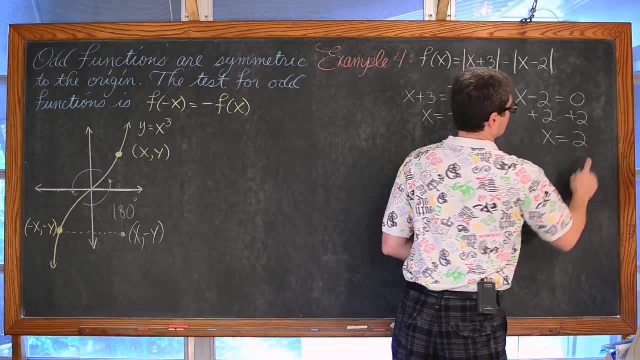 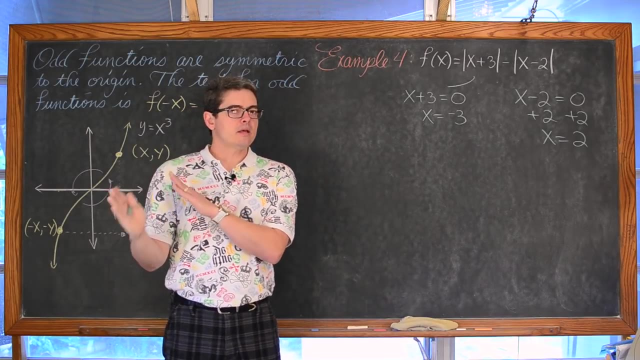 sides by three, I get x equals negative three, And when I set this equal to zero, I get x equals two. I want to try: if you think about the negative four and positive four, they were outside those values and I got opposite numbers. 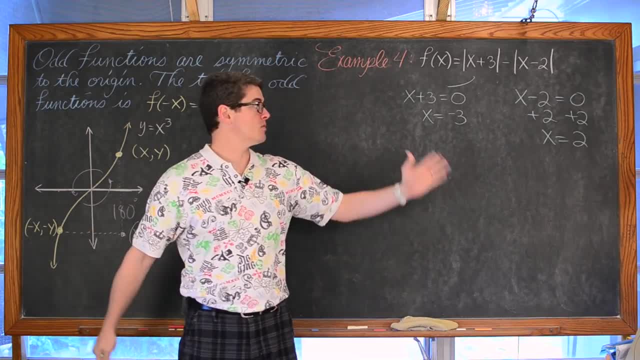 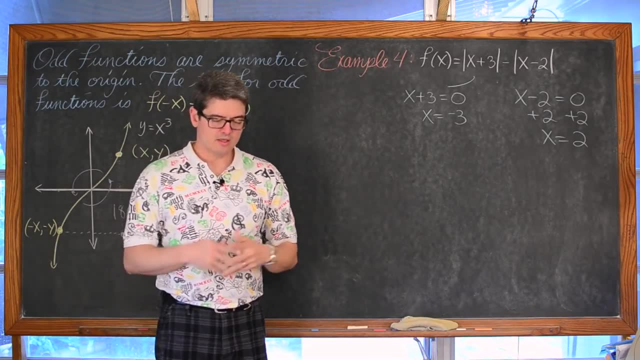 So if I try negative five and positive five or negative ten and positive ten, which are also outside those two x values, where the sharp bends of these absolute value functions- you know, if you graph them separately- occur, So Then I'm probably going to get the same kind of answer. 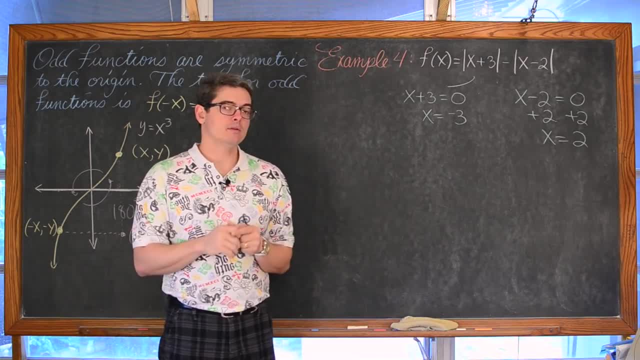 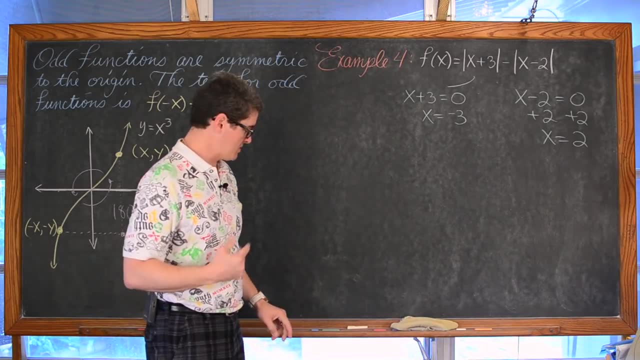 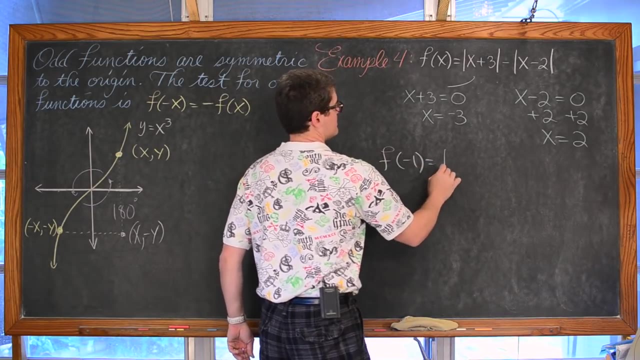 I want to try some opposite numbers that are inside this domain, if you will, Inside negative two and excuse me, negative three and positive two. So I'm going to try negative one and one. So we have f of negative one is equal to the absolute value of negative one plus three. 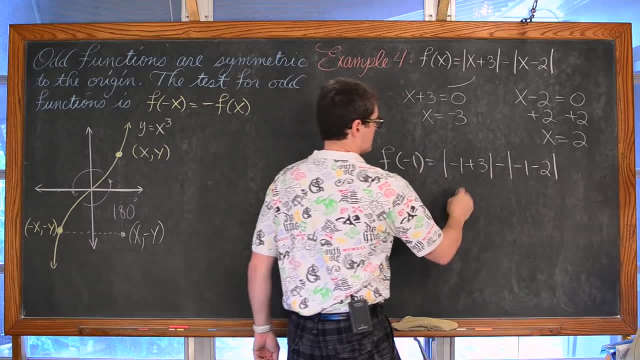 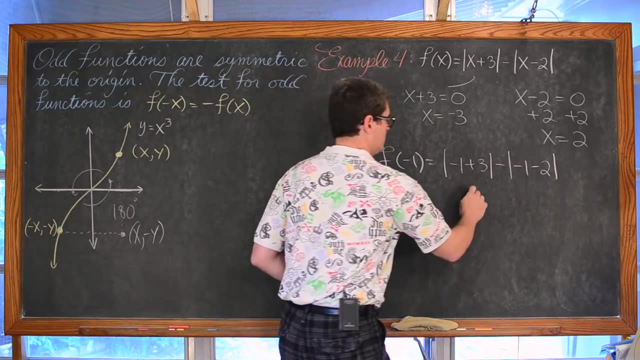 minus the absolute value of negative. one minus two And that's going to be negative one plus three. when you combine numbers with different signs, you subtract and keep the same And we'll get the sign of the largest number. So three minus one is two minus the absolute value. like signs, 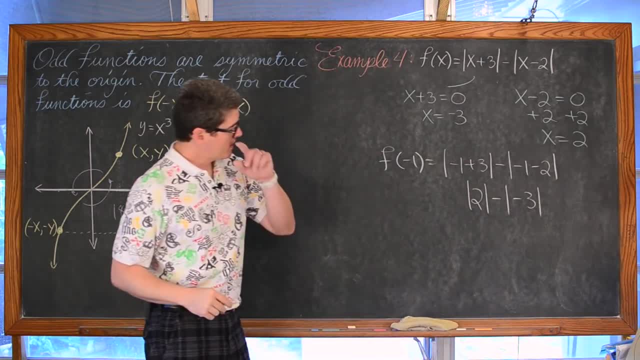 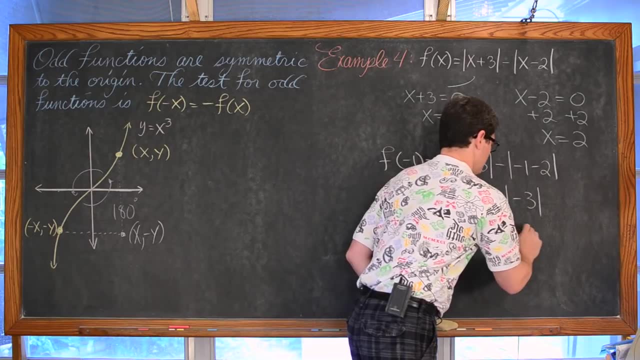 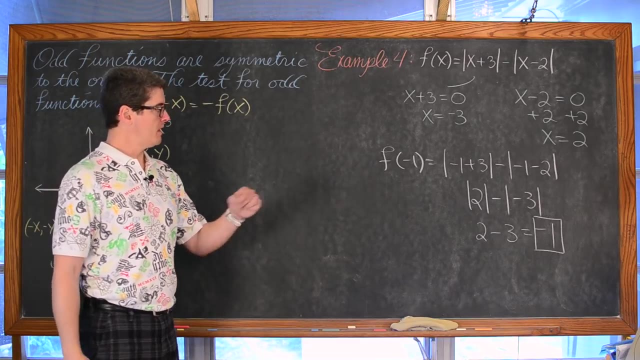 We're going to add those and keep the sign And we get two minus the absolute value of negative three is positive three And we get an answer of negative one. Now let's try the opposite of negative one, which is positive one. Okay, 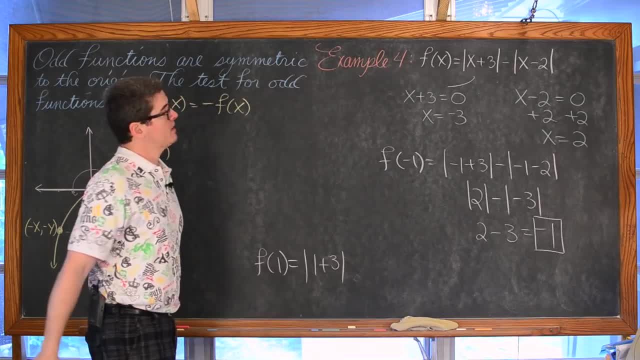 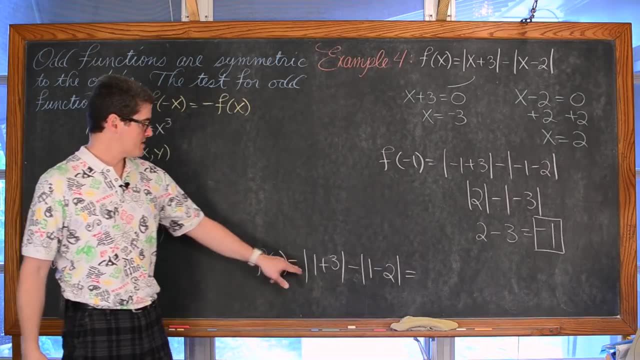 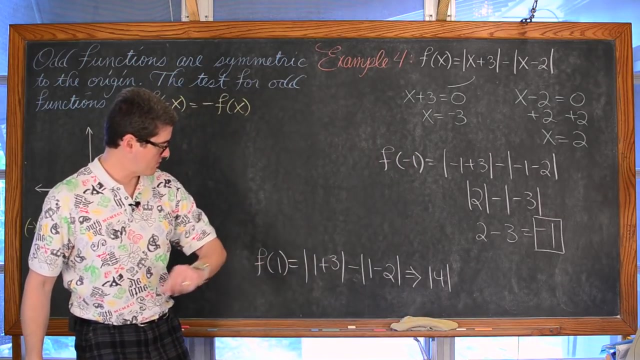 absolute value of 1 plus 3 minus the absolute value of 1 minus 2.. That is going to be 1 plus 3 is 4.. Sorry, I kind of ran out of work. I don't like to work sideways. Minus the absolute: 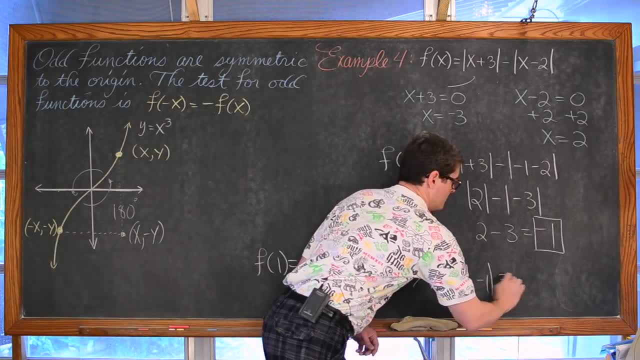 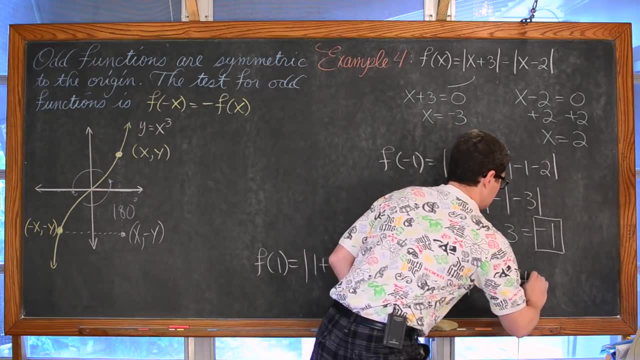 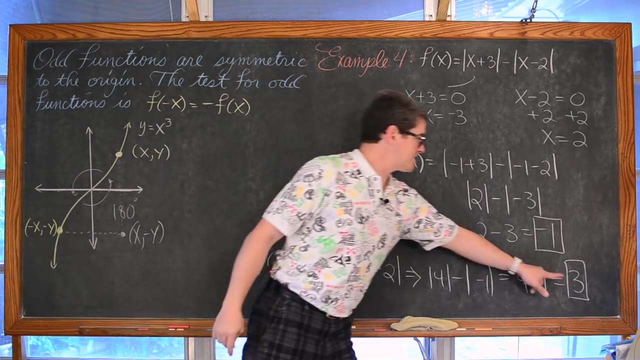 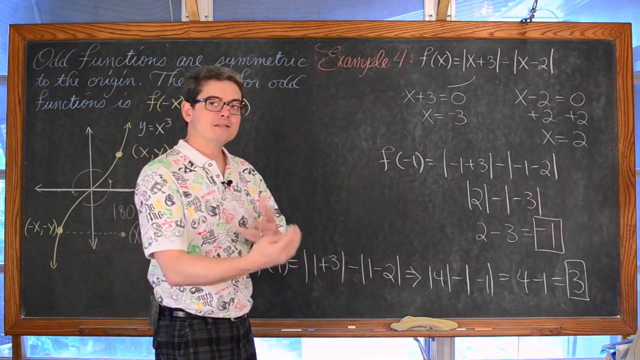 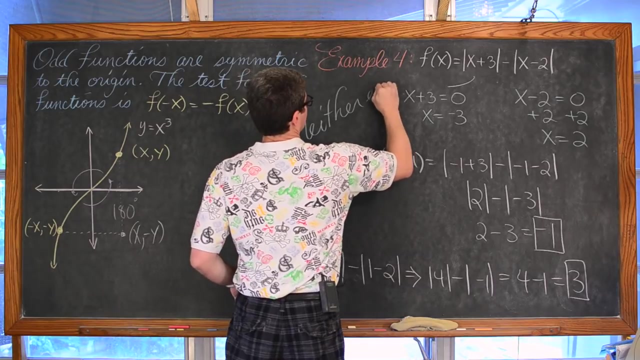 value of 1 minus 2, which is negative 1.. Now we get 4 minus the absolute value of negative 1 is 1.. We just plugged in opposite numbers and did not get answers which were opposites. So this is neither even or odd, Which is you know. it is ok, There is nothing wrong. 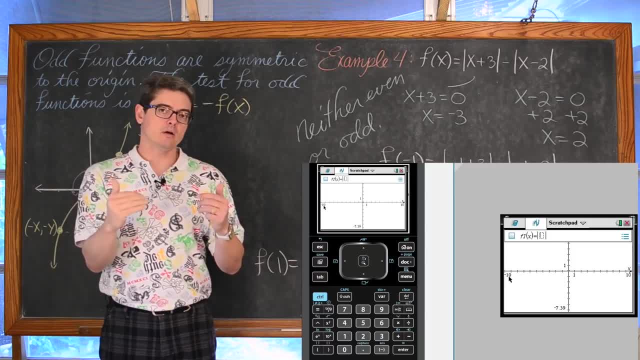 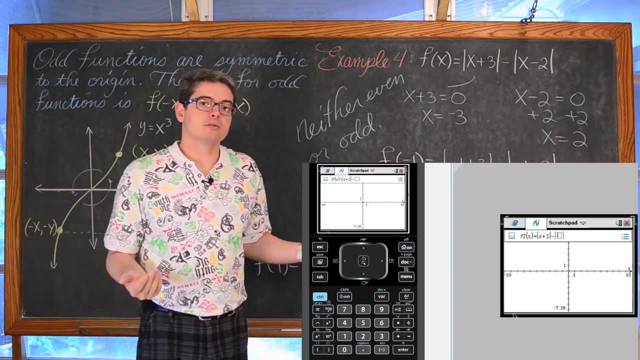 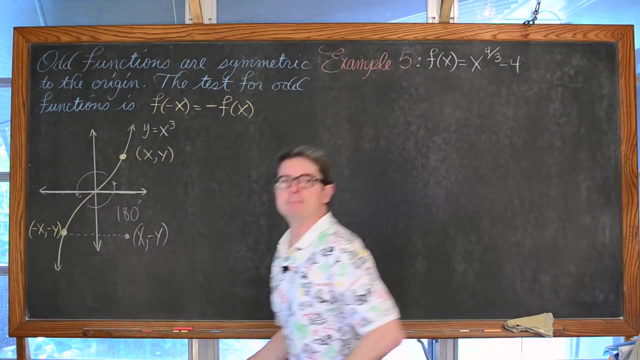 with that function. And, by the way, when I step off, I will show you what the graph looks like on a graphing calculator. It just means it doesn't have symmetry to the y axis, nor does it have symmetry to the origin. That is all. I got. one more example, BAM. Last example: We got f of x. 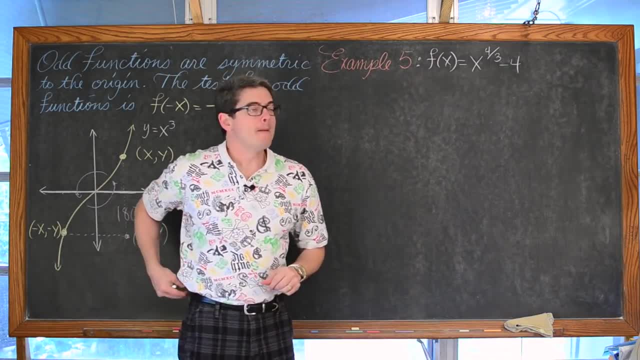 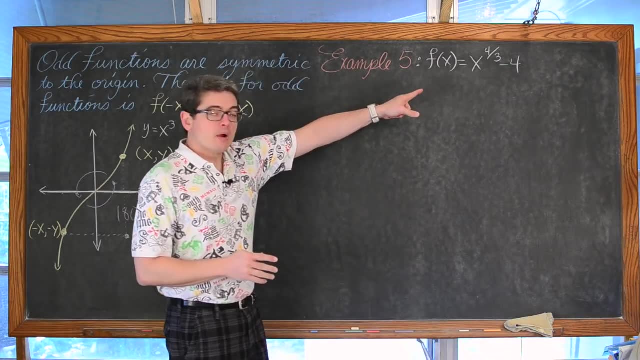 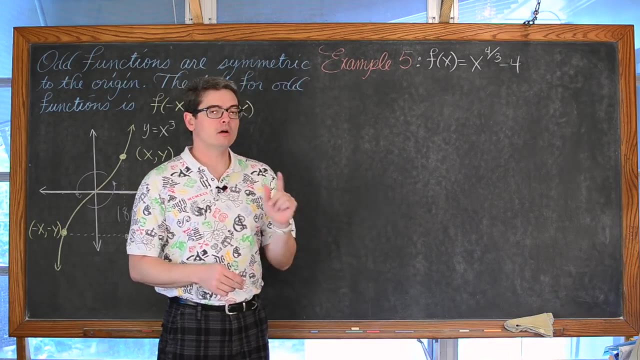 is equal to x, to the 4 thirds power minus 4.. We are going to be looking to see if this is even or odd. Now we have got a rational or a fractional exponent. I am not sure if you have had that in your studies yet or not. If you have, great. If you haven't, once you have been introduced. 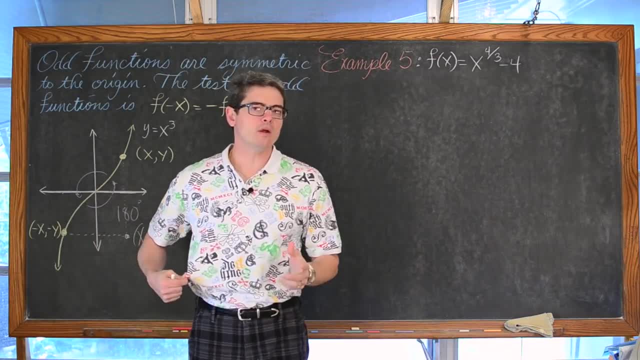 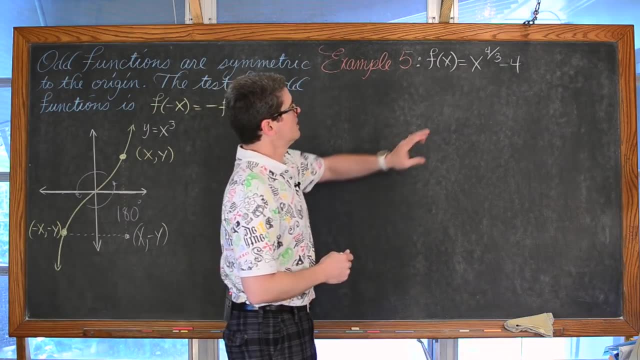 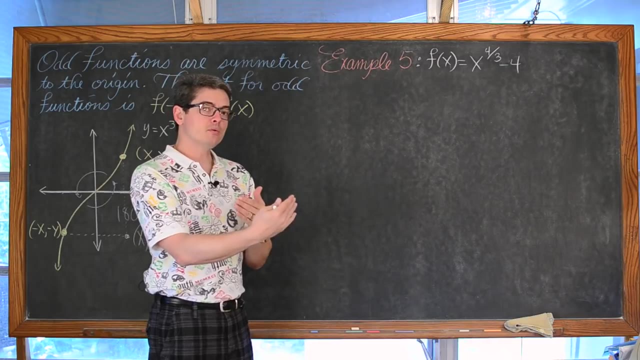 to them, don't avoid them. They seem a little bit weird at first because you are used to square roots and radical symbols, But working with rational exponents really makes work, when you have powers and roots together, much, much simpler. But I am going to convert this: 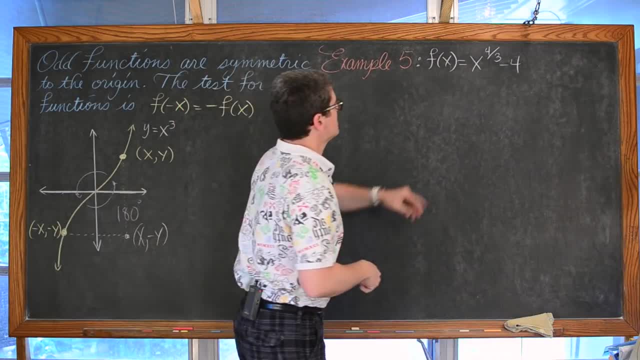 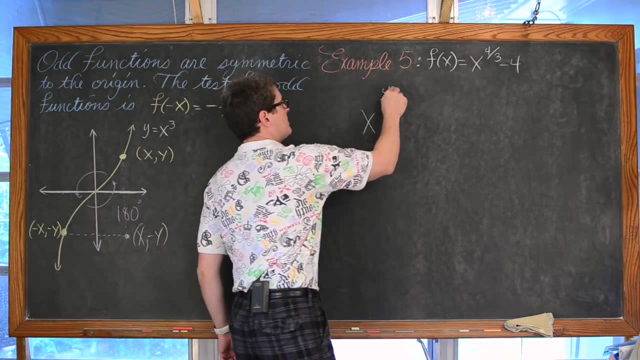 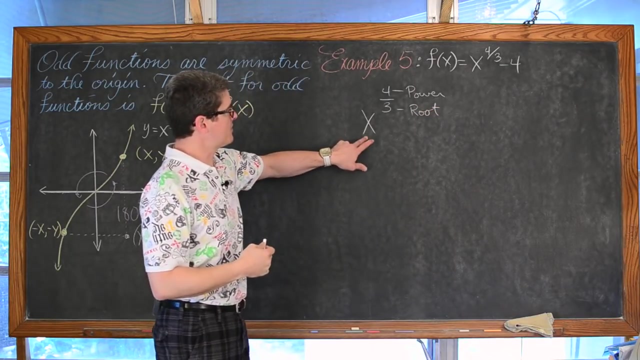 into radical form, Just to have It will. let you see it both ways. So when you have a base to a fractional or rational exponent, the top number is power and the bottom number is your root. So you are looking at something that is being raised to the fourth power and at the same time, you are taking 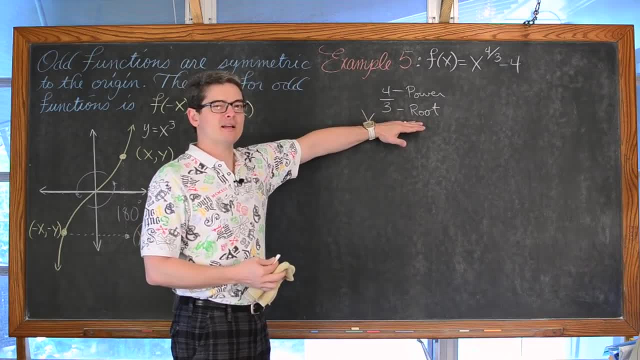 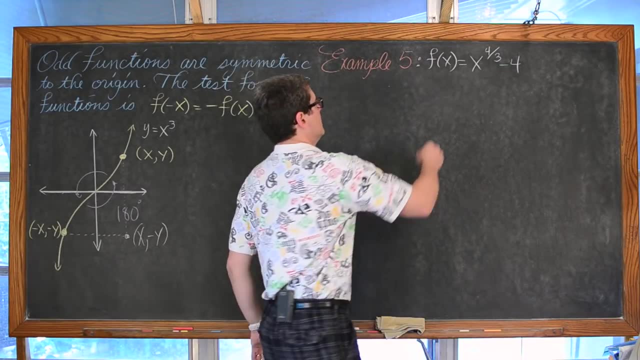 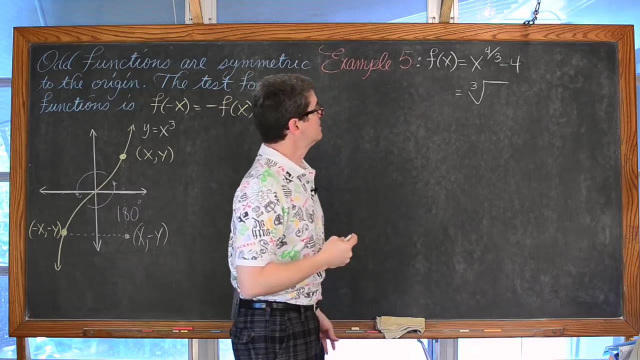 the third root of that value. If you are doing it mental math, I usually tend to like to do the roots first and then apply the power, So x to the 4 thirds. power is the same as the third root. that is the index of the.